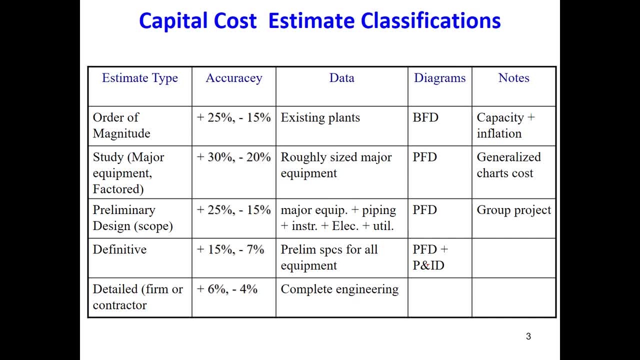 detailed and it can give us a lot of information, detailed information and it can give us the detailed cost that we have in the plant. so when? okay, for when? we can you know? like, use existing plant. let's say you are, you are going to fabricate, I mean construct, build up a refinery. 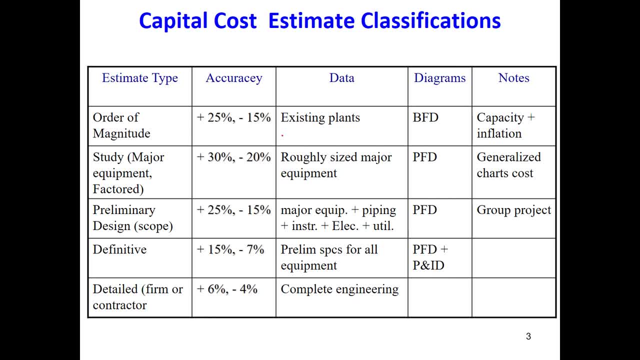 so you can just say in Qatar we are going to have a new refinery. so we know that in the area, like in Middle East, we have a lot of refineries in many countries. so there are some existing plant already. we can get some information about them, because whatever we will build will be not very far from 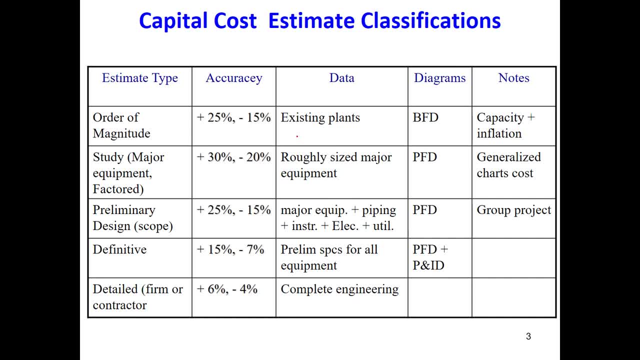 what is already existing in the region, because the properties of the oil that we have in Qatar is almost the same everywhere in the region. the climate is the same. I don't know like the expenses for workers, for operating costs, like all, are almost the same order of magnitude, okay. 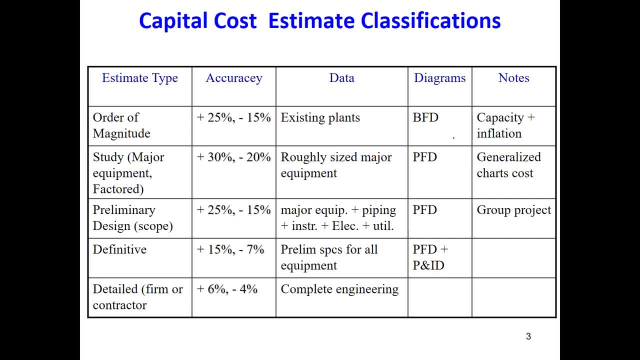 and then so we can use the existing refinery or plant with block flow diagram. we don't need to go through the details and estimate the cost of our refinery based on the capacity that we will have. so this kind of evaluation doesn't give us really a very accurate estimation of capital cost. it has an 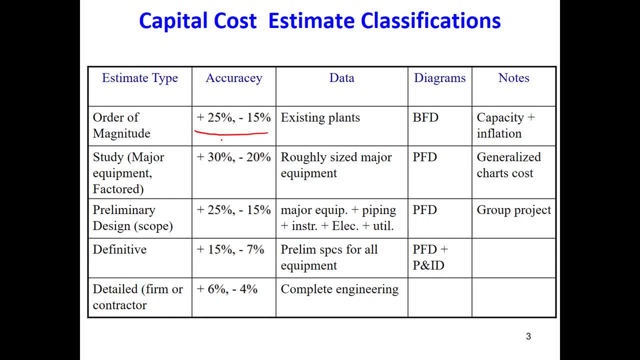 error between minus 15 to 25 percent. so whatever we calculate might be different from actual investment that we have and the accuracy will be in this way. we can also go a bit more details. use PFT process flow diagram and do some- we do- sizing for the major equipment. okay, reactors. 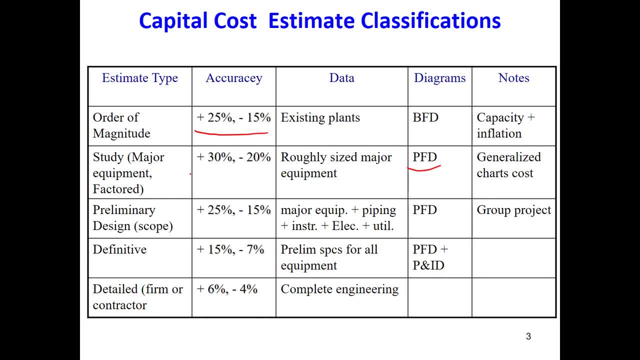 distillation column, those major equipment that we have and we just roughly size them. we don't need to go through the very accurate exact sizing, just roughly design and this can give us accuracy again between minus 20 to 30 percent of the final actual capital investment that we need to put and for 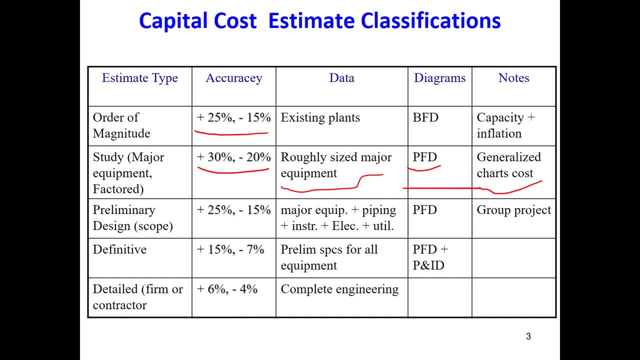 this we use some generalized the chart cost that we are going to talk about them later in this unit, a generalized chart cost, generalize the chart cost, chart cost cost that are produced already by some companies. then we can even go a little bit more details. okay, we can do the the sizing of different equipments. 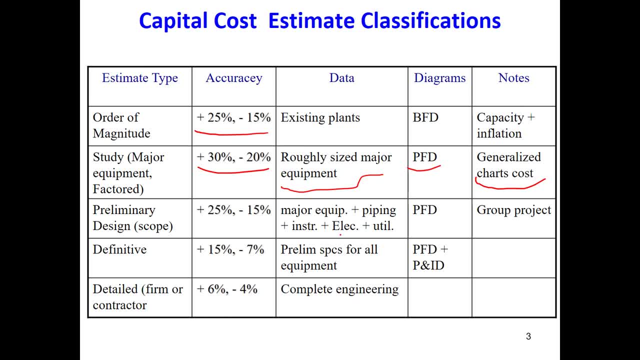 major equipments. we do some calculation for piping instrumentation, things like that, and we use the preliminary design. okay, again, it has still high amount of error or low accuracy, between minus 15 to 25 percent. we can go a little bit more detail, which is using the all the information from PFT and PNID. 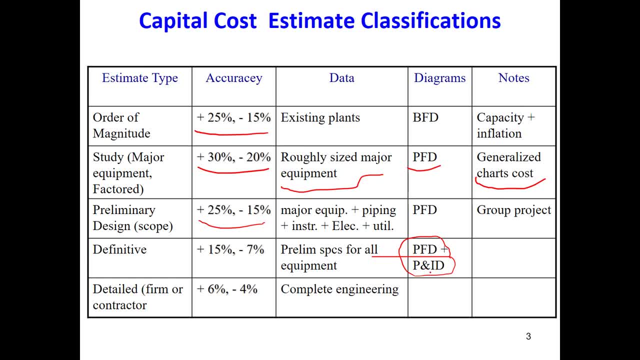 process flow diagram and process pipe and instrumentation diagram in. when we do this, when we use this kind of diagram, we use all the information, all the details, We do the design and finding the specification of almost all the equipments, especially the preliminary equipments, And when we do this kind of calculation we will be really close. 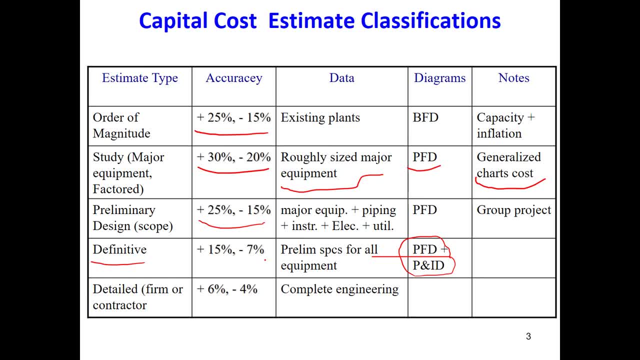 We will be very close to the, to the actual investment that we need to put. So, all these methods, they give us some idea about how much money that we need to put. But, as I said, we have this kind of accuracy- low accuracy- between minus 20 or plus 30.. 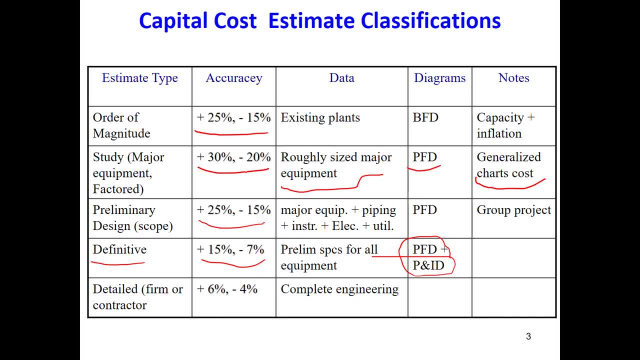 It means, whatever we calculate from here, it might be either 20 percent less than what we really need to put, or maybe it is like 30 percent more than what we really have to put already. OK, so that's that's the issue. But here we get really good estimation of the investment that we need to put. 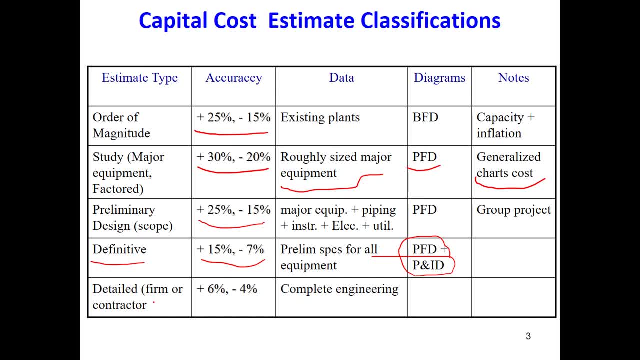 OK, And we can still go further. OK, go further and do a very complete engineering job by considering all the calculations here, plus calculating the labor that we need to do, different contracts that we need to do like operating costs that we have, task modulation costs, taxes, almost all the things that will be involved in the process. 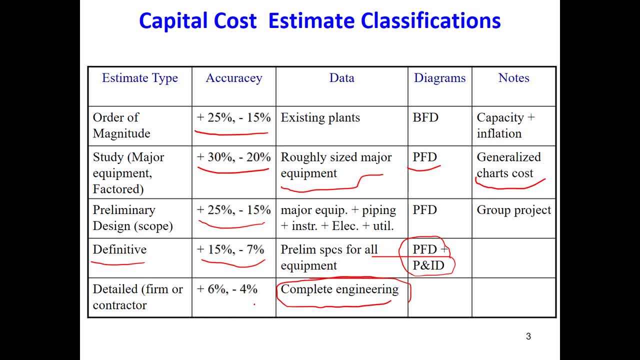 that we will be doing. So we will calculate and we consider, And at the end what we get it is the estimation that is very close to our actual final investment that we need to put between minus, almost like minus, minus and plus. five percent error between what you calculate and the actual one. 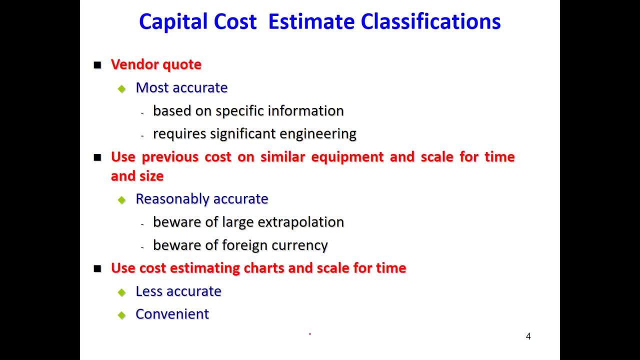 OK, so for the cost estimation, OK, For the cost estimation, We can use different sources. OK, let's say, let's for now just talk about the equipment, the equipment that we have in the plant. OK, and we need to find the cost. 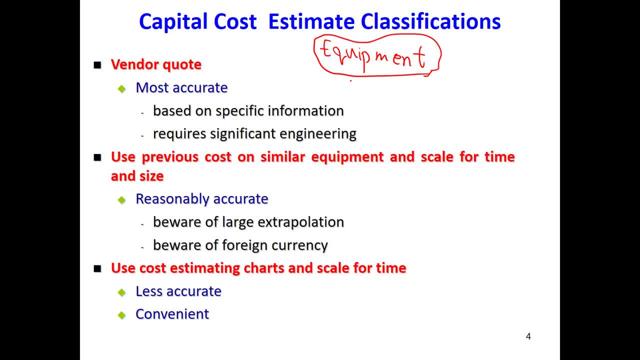 Let's say we have heat exchanger, heater, reactor, distillation column. We have many equipment. We just need to evaluate the cost, All right, So how we can find the cost of this Equipments? OK, we have different sources. 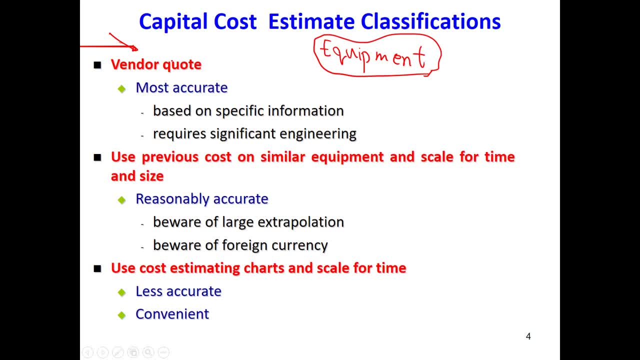 First, very simple Wonder code. OK, you want, you want to buy a heat exchanger compressor. You know like in Qatar, we have few wonders that they said they import heat exchanger or pumps from, you know, other countries. 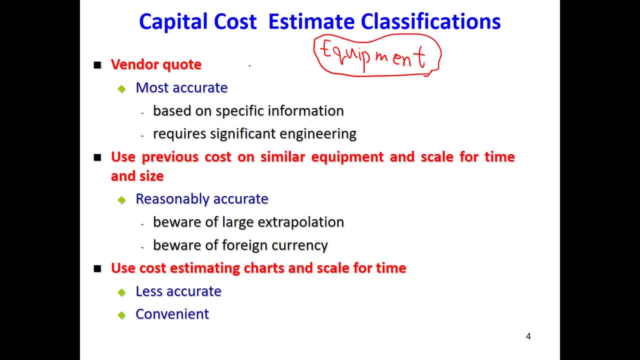 You just call them and you tell them: I need this compressor, I need this heat exchanger, with this specification, And, and how. I mean like, please, please, give me a quote, How much does it cost? So, like what they do, they both look at the companies, the suppliers they have. 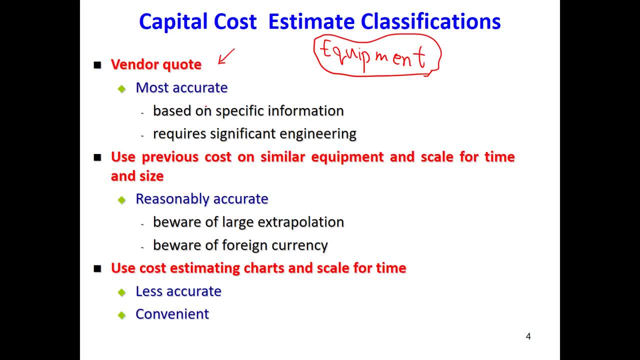 They find you a list of companies that they can, you know, produce this, They can provide it for you, And then they give you a very accurate price of that equipment. The updated price is a price for that. you know, like up to that day. 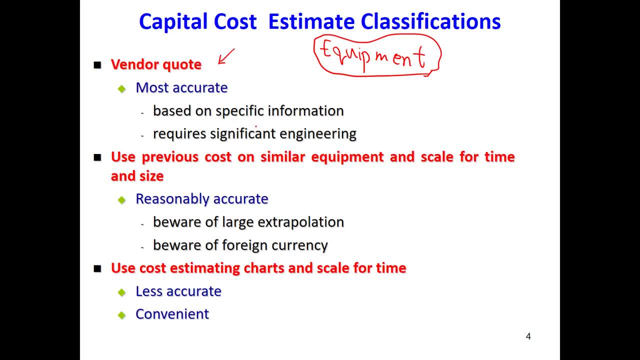 So it's a very accurate way of finding the price. And for that, for that, when the wonder is want to give you the price, he will ask you for exact, specific information: What will be the size, What will be the load? 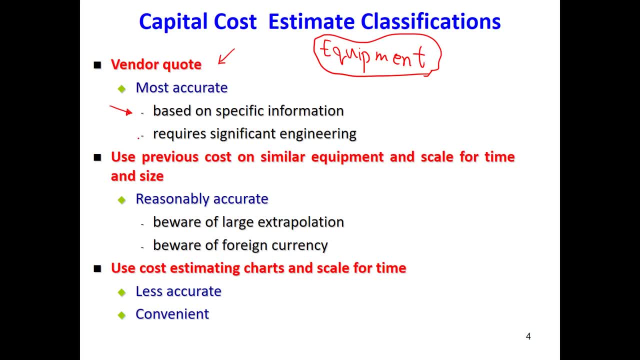 The heat beauty. You know all this specific information, the material, the operating pressure, temperature, all those information will be asked from you. And, yeah, All We, We can use the previous cost for the similar Equipment and scale them to the time and size. so 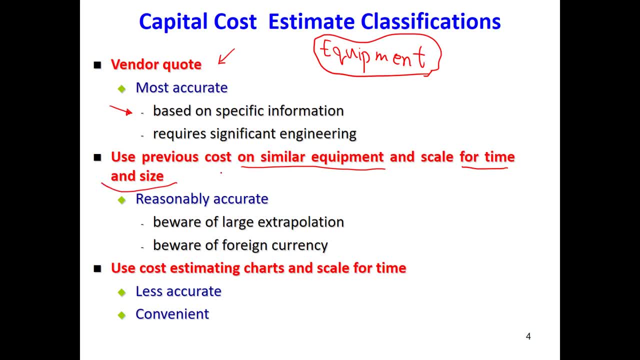 We can use. another way is that we can use some charts, some tables, that is, that list the price of different equipments with different size and different years. in previous years, Let's say. we have many charts like that that. you will see some, Some of them. 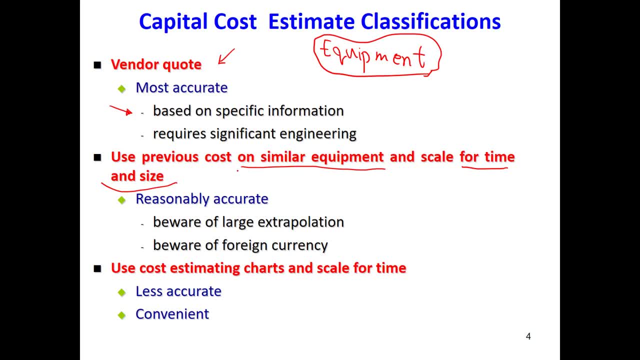 I mean chart or equation. So what are those? equation? So let's say we know that the price of a heat exchanger that was used in the refinery, in one of the refinery in Qatar in 2005, the price of that is exchanger. 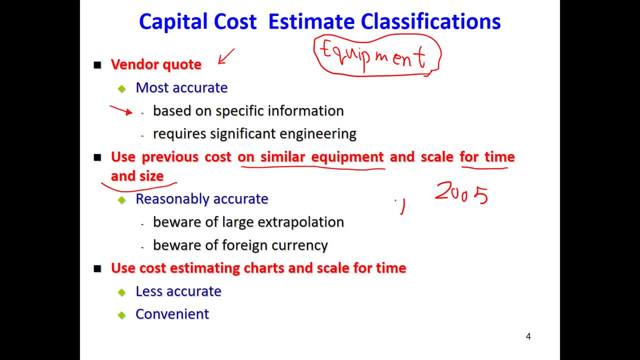 In 2005.. For the heat exchanger that had the surface area- Surface area, You know, is one of the most important parameter in the design of heat exchanger- The surface area in 2005 for the surface area of 100 square meter. 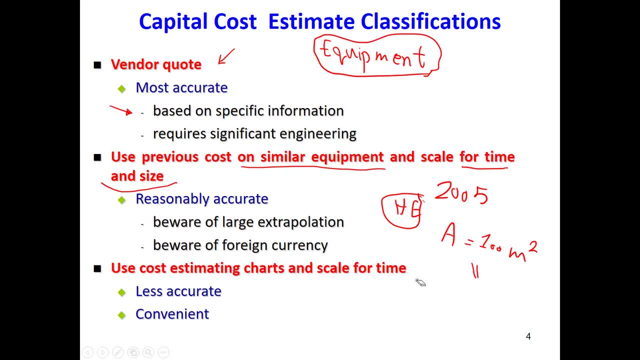 The price was. The price was, Let's say, I don't know. Let's say 10,000, $10,000.. Okay, Now that we are in 2020.. And If I want a heat exchanger that has 200 square meter area, what will be the price? 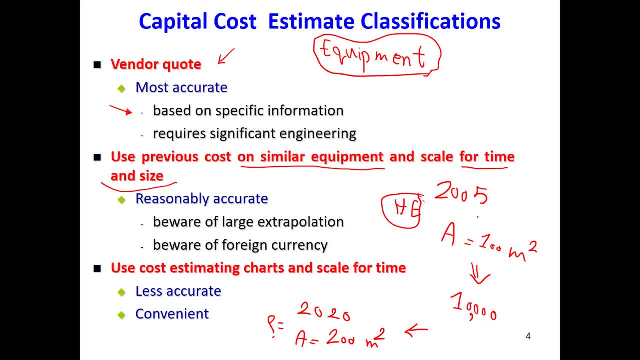 There are equations, There are some factors that relates this to this information to each other. There are some equations that we can use And we can say that, okay, if in 2005, the price was this, in 2020, we will. we just need to multiple that number by, by a factor, by indicator. 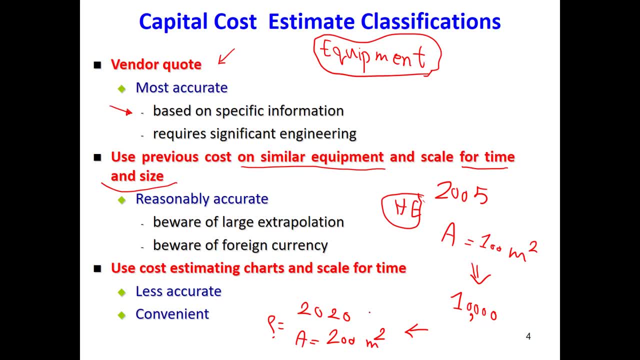 Those indicators are available in the internet, The company that we do it, And you just easily calculate the price of that equipment. So this method that we will see in the next slide is kind of is reasonable. Accurate is not like wonderful, but it still is a very good estimation. 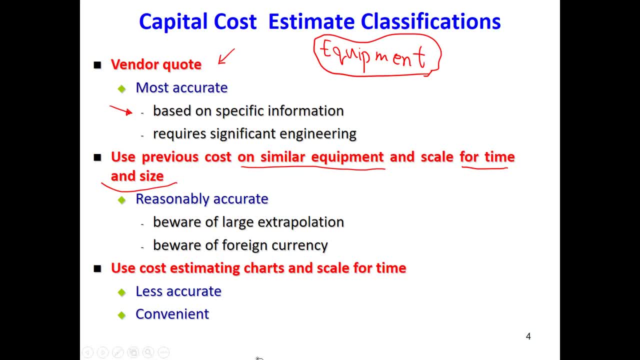 We is very quick to be, We will save some Some. Sometimes, you know, like to do the calculation. but we have to be careful that all this indicate, or the factors that we use, They have a range of application. We cannot just say, using a factor indicator for a heat exchanger that has a range of 100 to 500 square meter area to a heat exchanger that has a 2000 square meter. 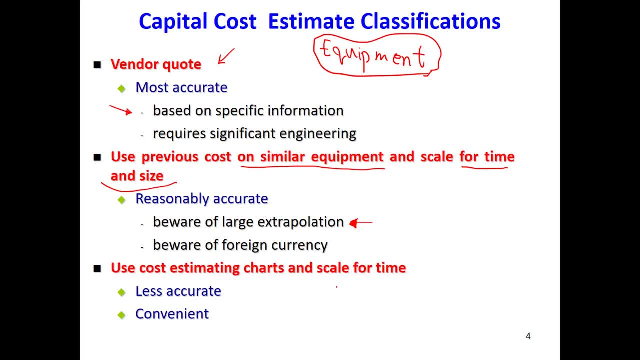 Right. So extrapolation has to be done carefully, Or So? Also, as I said, here we use some equations, Here we have- We cannot use some- Some Charts as well. Okay, That are less accurate, But they are convenient. 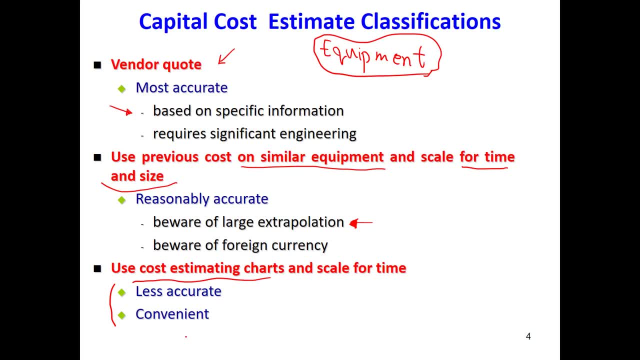 You know Like they are not very bad, But although they are less accurate, Then Then What we have? Okay, So this is one sample of equation that you will also see, one example how to use this equation. So, As I said, 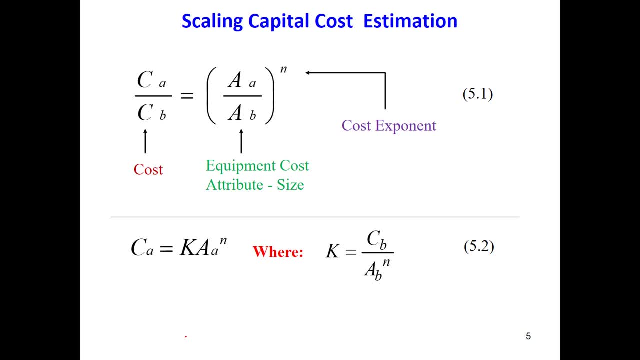 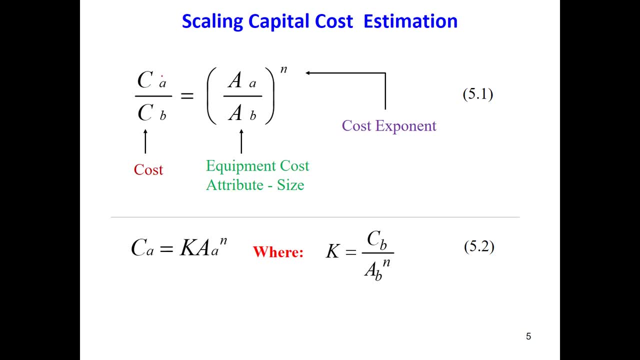 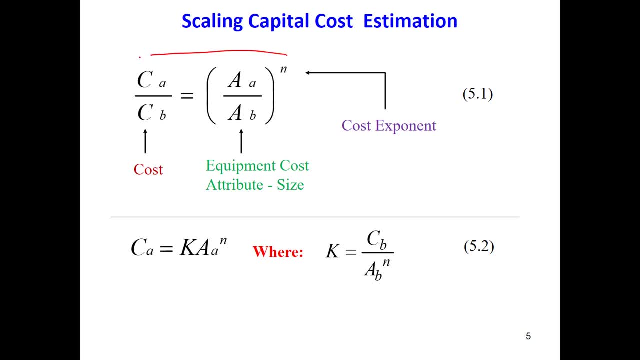 Okay, Okay, This is called a scaling capital cost estimation. This equation is a scaling capital cost estimation. How we use this equation. Let's say we have the price, The cost of a heat exchanger. In cost of heat exchanger that has a surface area of 100 square meter, we have the cost. 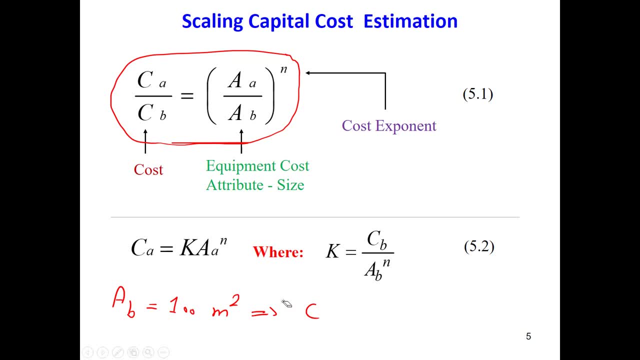 okay, let's say in this year we have the cost in this year for this heat exchanger. that is, let's say, five thousand five thousand dollars. now, if I want to buy a heat exchanger that has 250 square meter, okay, what will be the cost? this is the typical question that we have. 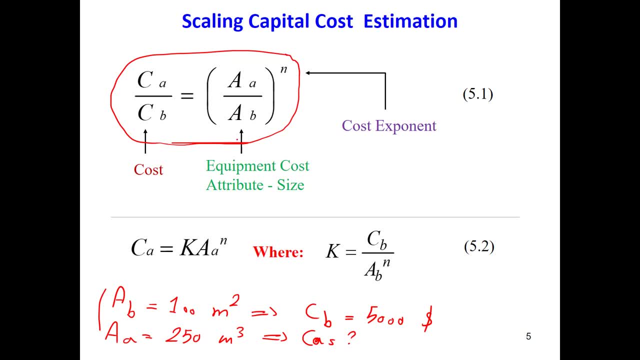 in to use this kind of equation. so we can use this equation. we have the surface area, okay. the second one, the last one that I want is 250. this is 100. I have the previous cost, the cost for 100, which is 500. I just put in this equation. I will find the cost of my heat exchanger. 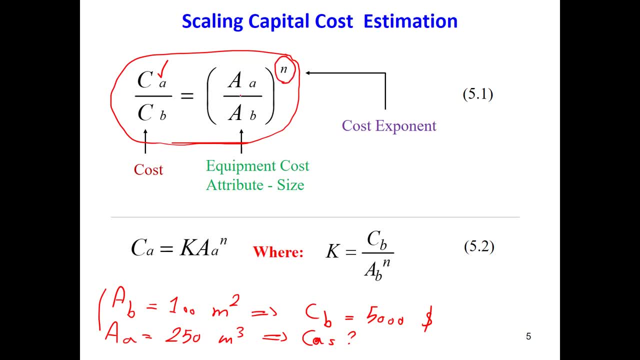 so the most important, The most important parameter here is this N. here we call it cost exponent. So this cost exponent is usually about 0.6.. OK, in the next slide you will see that. And yeah, like this, this is the equipment cost attribute. 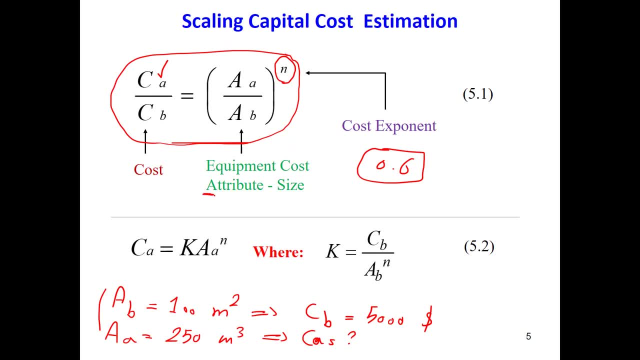 OK, the A. we call it equipment cost attribute. That's why it's wrong with A. The C is cost OK. so this A sometimes can be the size OK, it can be, for example, for heat exchanger. it can be area, surface area. 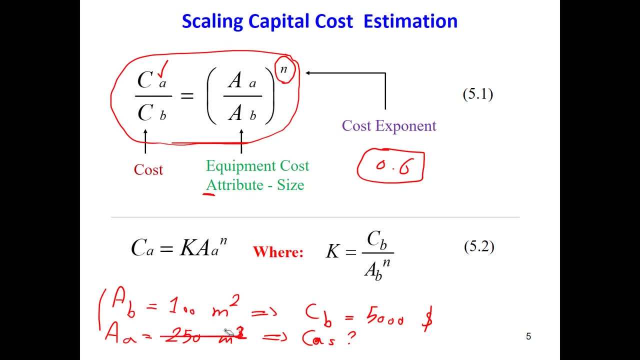 So let me correct this here, please. So for a heat exchanger it can be area It can be. for a pump, That can be the power It can be, I don't know. for a fire heater It can be the air. 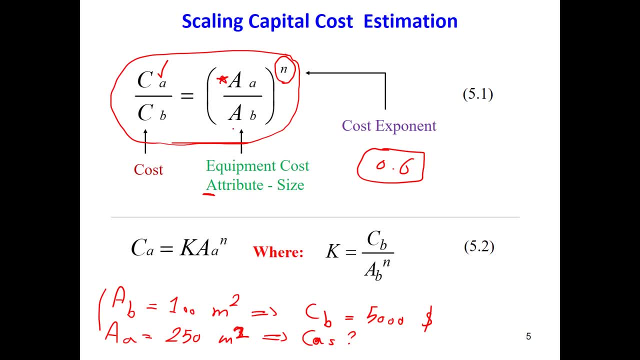 It can be the heat duty, the amount of the fuel, So it can be any parameter. It's not necessarily the area, OK, but since it's showing with A, I just give you an example of area. But this is called equipment cost attribute. 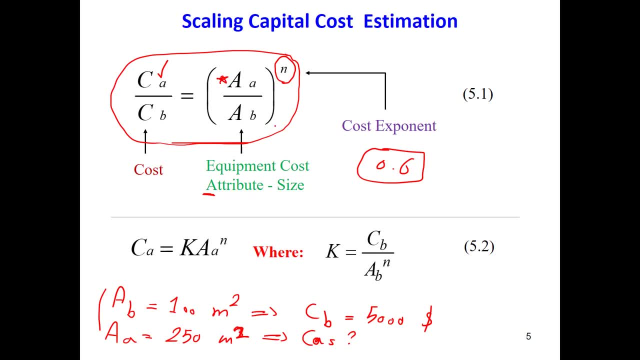 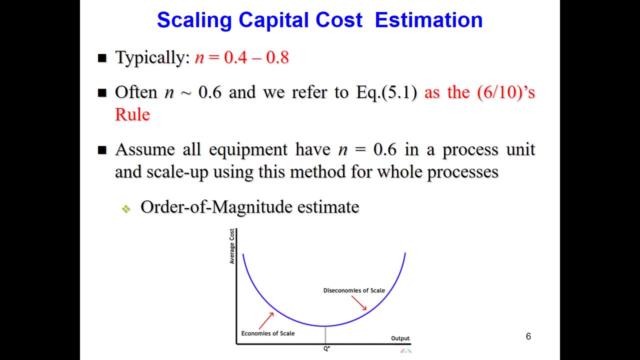 It can be any parameter: capacity, flow rate, power area and so on. OK, this is OK. N is usually between 6 to Yes. N is usually between 6, 0.4 to 0.8.. 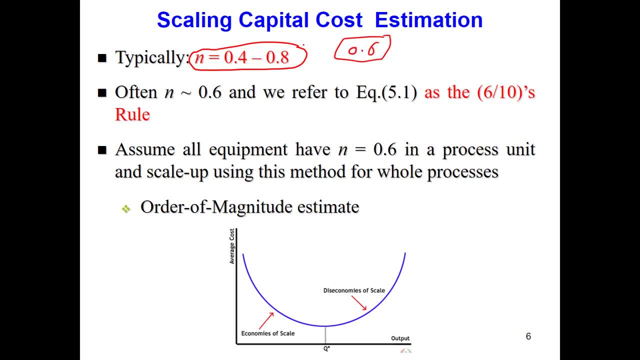 And a value of 0.6 is a very typical value that they use it in many, many places. Then, as I said, 0.6 is one of the typical value and they call it when we use 0.6.. 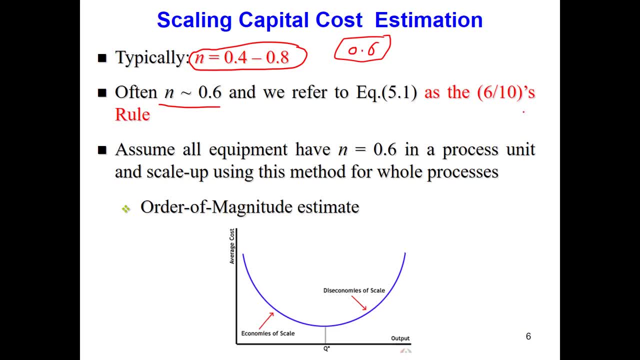 They call it the 6 over 10 zone or 0.6 zone rule. They read it in this way. So most of the time we assume that all the equipment they have- I mean for all equipment- most of the time we consider 0.6 when we are going to. 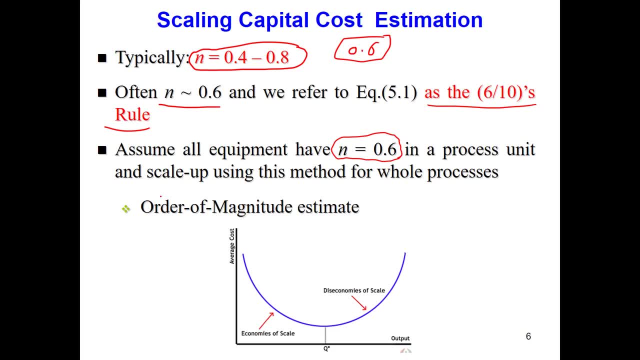 When we are going to estimate the cost of the equipment. And don't forget that When we use this equation, it's just kind of order of magnitude estimate. It's not, It's not really, you know, very, very accurate. 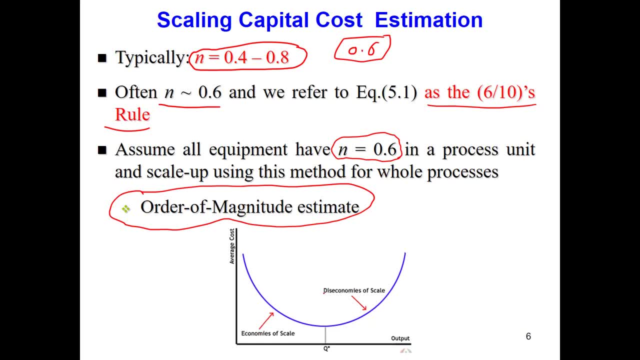 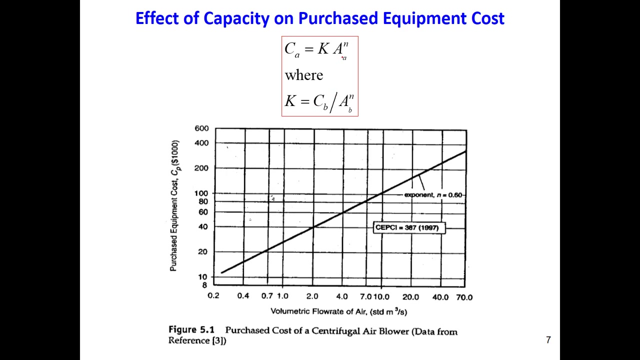 This is kind of order of magnitude. This is not OK, This is not very important. I will show it more. Just show you one example that you know, like how the cost and the capacities are related. So OK, We, we have most of the time. 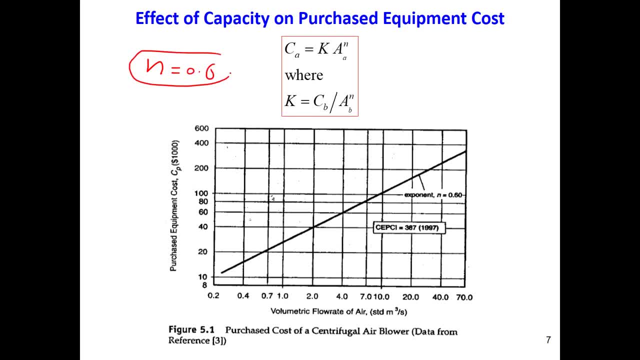 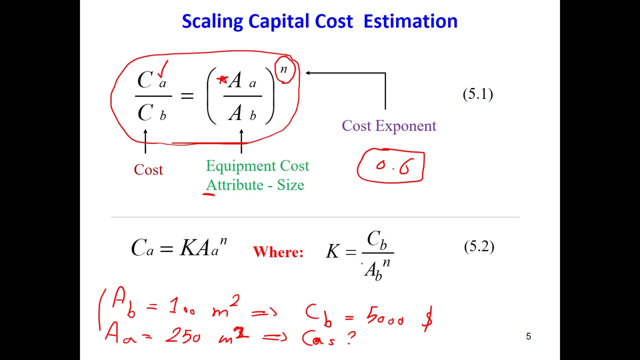 And, as I said, and 0.6, or sometimes we have such a such a, such a curve. you know that, that, what is this curve? So here what we have done instead of: we can simplify this equation and we can extract, We can put CB and ABN all together. 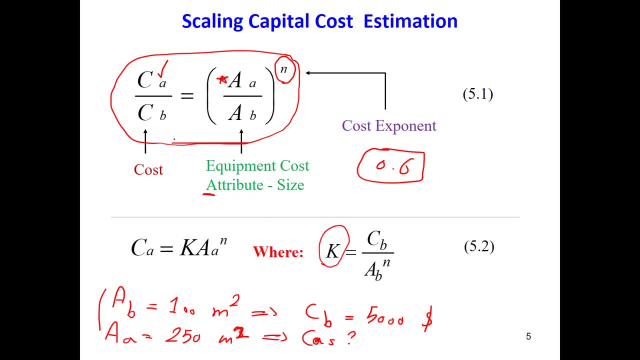 And we call it K the coefficient. OK, So then we, instead of using the above equation, we can use this equation, CAKAN. OK, So K is a constant, N is a constant. So then A, this A and C, they will be the variable. 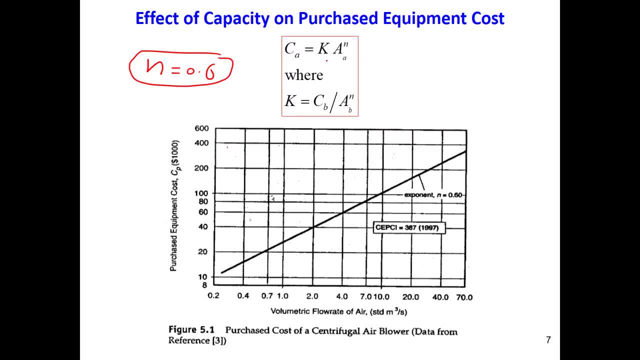 OK, We can do, We can plot, We can plot CA versus A In this such a curve. OK, If we do it in the logarithmic axis, OK, We can have. We can have a straight line that has a slope of 0.. 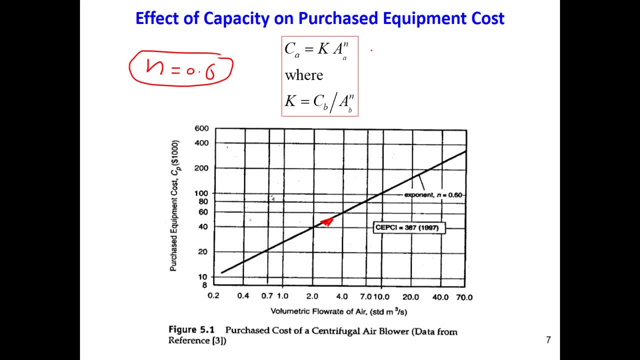 N, which is 0.6,, for example, How we can do it. If you take a LN of this equation, you will have LNCA, LNK. OK, So it's going to be OK. So here is the LNK. 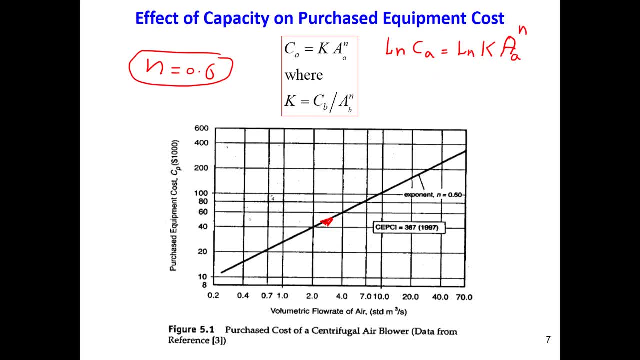 OK, AAN, Yes, OK. So, based on the properties of LN, this will be LNK plus LNAA. power N, Again based on the properties of LN, So it will be LNKN times LNAAA. OK, So, after this part of the equation, 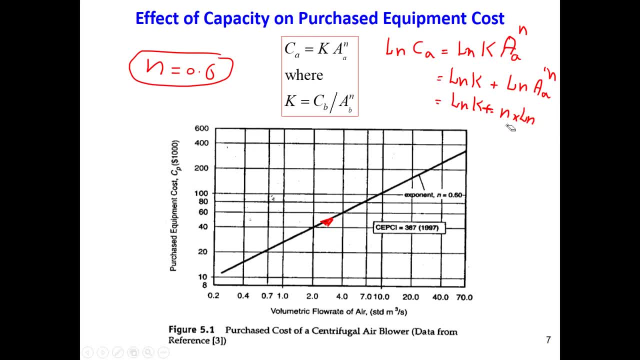 We have the result AA. okay, so this is your x-axis, this is your y-axis. okay, this is your y-axis here. so what you have? you have now a line y equal to nx plus ln k. okay, so this is your y-axis, this is your x. so this, this curve, is based on logarithmic. 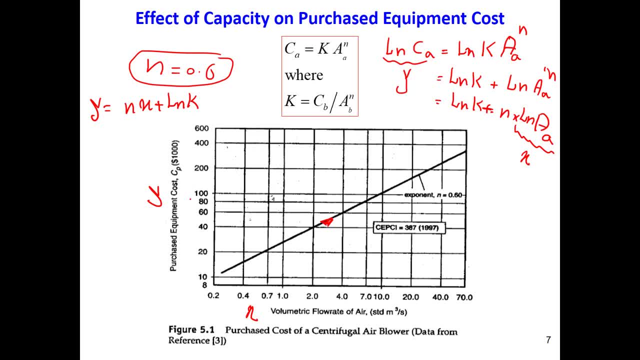 logarithmic axis. okay, that is a straight in the logarithmic axis is a straight line that has a slope equal to n. okay, and the intercept is here: k. this is your intercept. okay, ln. k actually, okay. so, no, no need to know this. this details. I just wanted to know to tell you why we have this line, this. 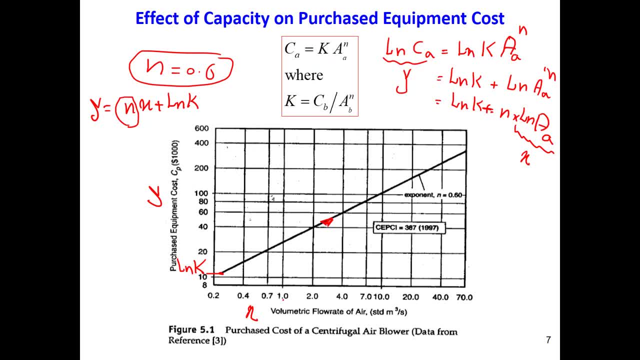 straight line, because we use this equation in logarithmic axis. so like this is for the centrifugal air blower that, for example, if I give you, if I give you is already you know. like you don't need the initial condition, let's say you don't need to know what is the initial condition, what? 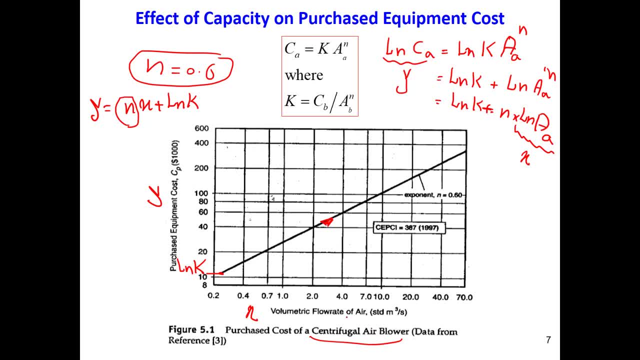 you how you use this. you, let's say, I give you the area of the flow rate of the centrifugal air blower that you need to purchase. let's say, I give you the flow rate- seven cubic meter per second. seven cubic meter per second, and you just go to this. 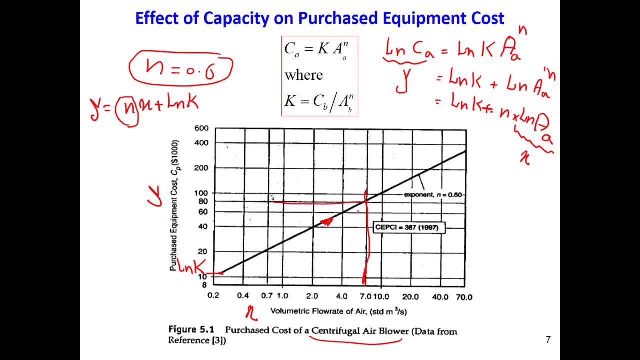 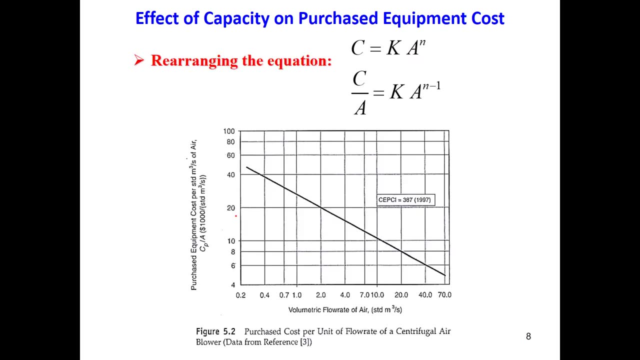 curve up to here and you go. you go first vertically up until you reach to the curve to remark that point, and then you go horizontally and find the price okay. so it's very. this is how simply we use this curve. or okay, if instead of you know some, some other charts, some other curves, instead of plotting C against N. 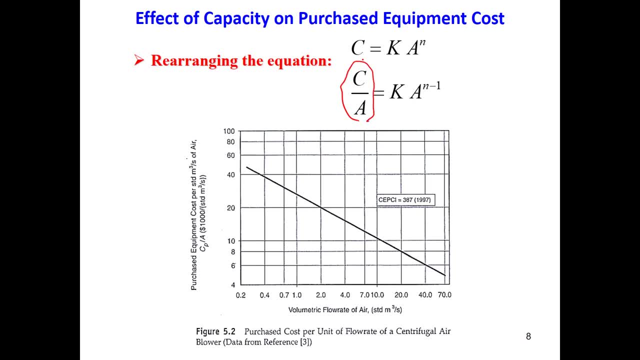 they plot C divided by C versus a. they will plot C over a versus a. so, in that case, what you need to do, you just need to extract one a from here that you will have a n power minus 1 times a. okay, a k times a power n minus 1 times a. 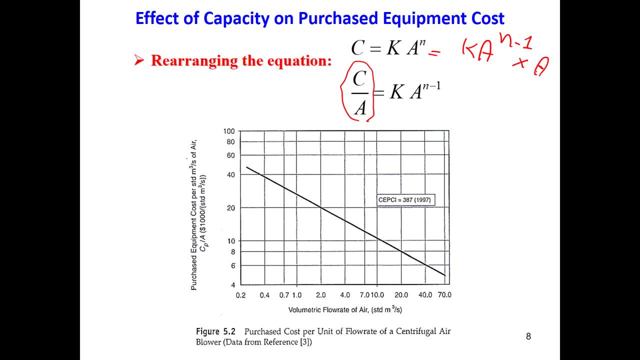 you just need to put take a to the other side, then you will have such a: CA is equal to k a times n minus 1, so this will be your X. this will be y in logarithmic axis, actually. that's why now you have a line that has the slope n minus 1. okay, if you put n 0.6, you will have a line that has the slope n minus 1. okay, if you put n 0.6, you will have a line that has the slope n minus 1. okay, if you put n 0.6 you. 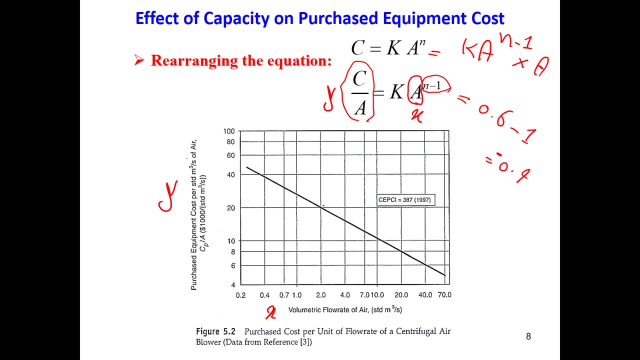 will have a slope minus 0.4. that's why this line is declining. it has a negative, negative slope. okay, so instead of C, now we have CA. for example, in previous chart we had cos. now we have what we have: cos per the volumetric flow rate, cos per, as I said, a can be area, can be volumetric flow rate, can be mass. 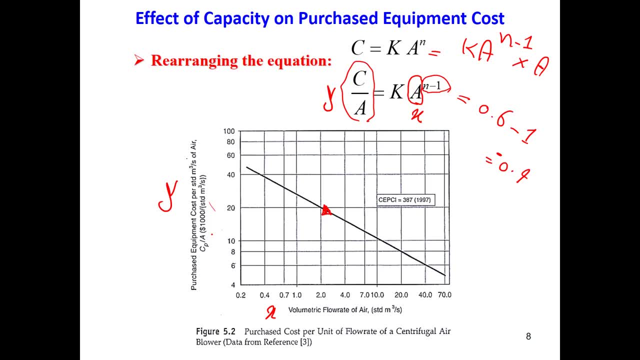 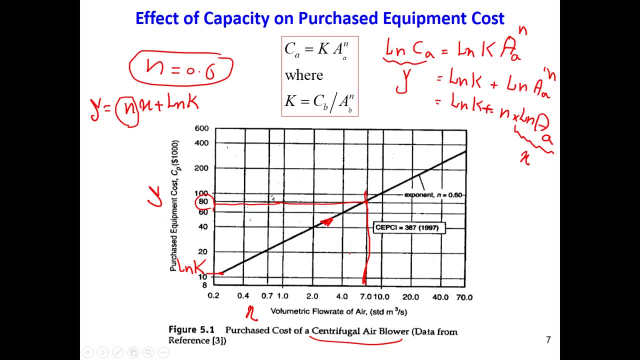 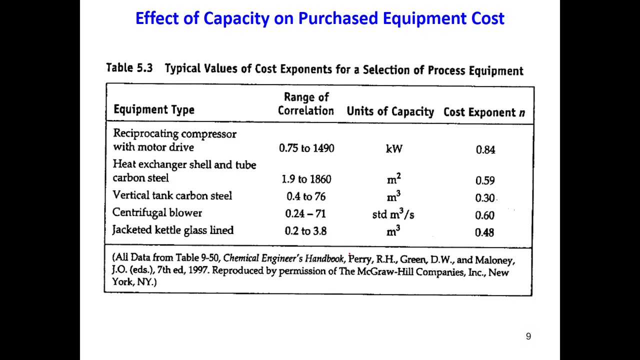 flow rate can be. power, depending to the equipment, is different parameter, so you have the cost per flow rate. okay, so here you have X axis, which is your volumetric flow rate. here you have the cost per volumetric flow rate. so we can have these two type of charts: the first one here and this one then. okay, in this. 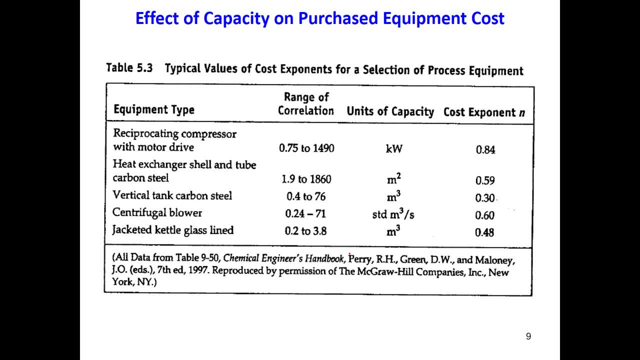 table. this table give us some additional information for, let's say, for n, okay, for n. sometimes we need to, sometimes we need to know what's the exact n. there are curves, there are many, I mean. there are tables like that that can give you the value of the n, for example. this is one example of those. 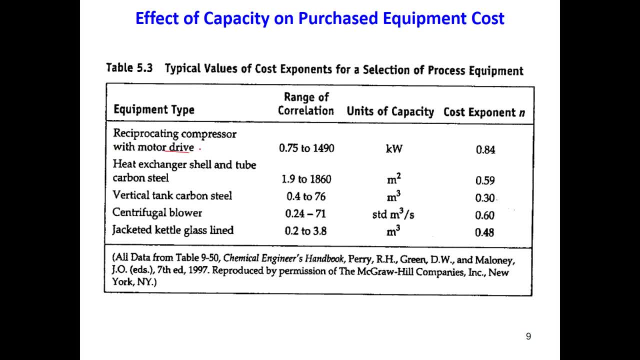 table that we have, for example, reciprocating compressors with motor drive for the capacity in kilowatt in this range- and is this much for I don't know- vertical tank carbon steel that has a capacity between 0.4 to 76 cubic meter and that you have. 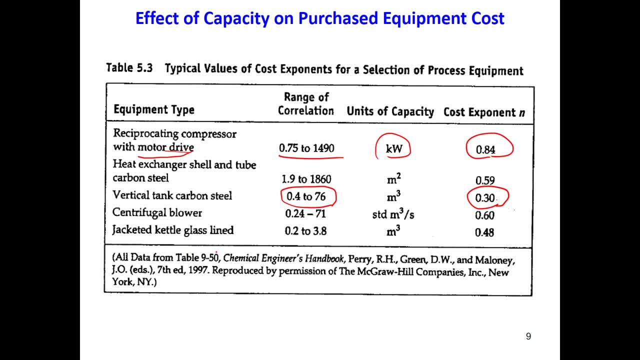 to use. is this one for jacketed cattle grass line. okay, that has the cutter is like for boiling something usually. so that has this can this much capacity in cubic meter. the end that you need to use in that equation will be 0.48, so we have different type of curves like that, that that. 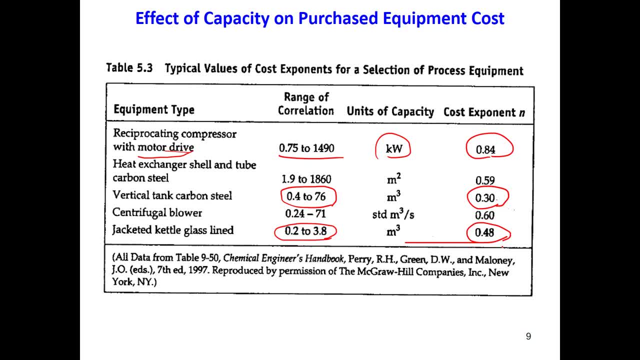 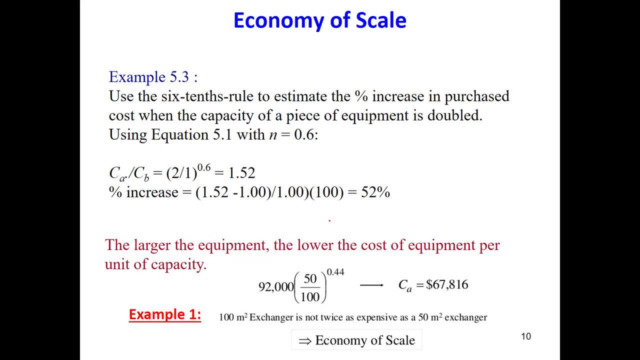 we usually use to. I mean different terms like that that we can use to find n for the specific equipment with a specific capacity, like, like what listed here. okay, we have an example here. please have a look at this example for a few seconds and then we will solve it together. 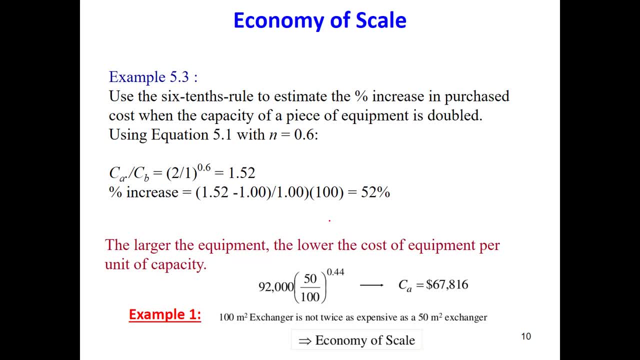 so okay. so, uh, it's a very simple uh example that, uh, I'm sure most of you could already find the answer. Oh yeah, use the 6 tenths rule. What does it mean, 6 tenths? It means n equal to 0.6.. 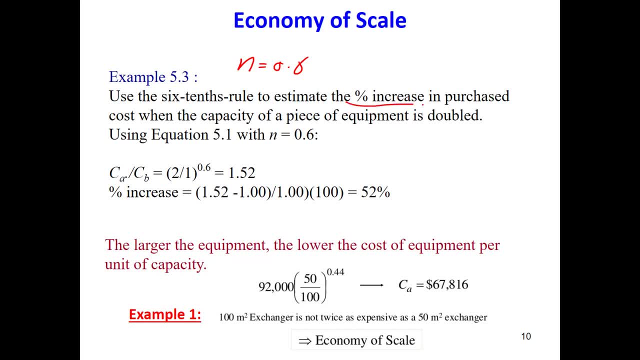 To estimate the percentage increase in the percentage percentage cost when the capacity of the piece of equipment is double. So we want to calculate the price of a piece of equipment that we don't know. what's equipment, we don't care. The only thing that we know is that the capacity, let's say the flow rate. 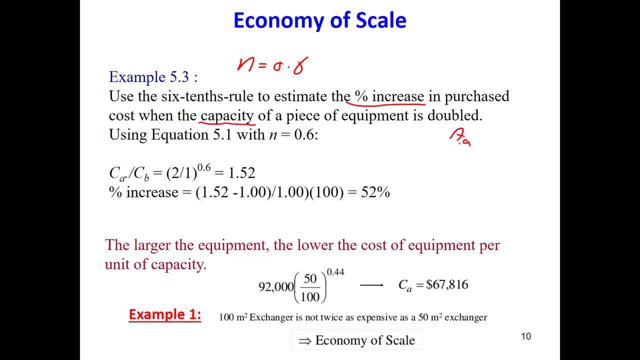 the power, whatever it is, is double. It means AE over AA over AB is double is 2.. Okay, so we have this equation: CA over CB is AA over AB and power is 0.6.. So what we will find here? we will find CA over CB is equal to. 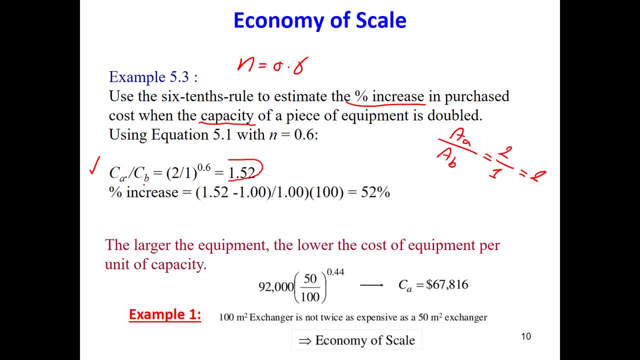 from this equation we will find 1.52.. Okay, so Before it was 1,. okay, when the capacity was the same. if you put the capacity 1 here, 1 over 1, give you CA over CB. 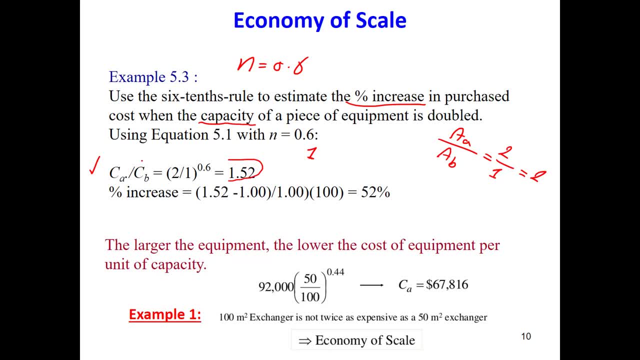 Okay, before that the capacity was the same, So this ratio was 1.. Now this ratio is 1.52.. Okay, so how much difference there is? how much percent? to find the percent we will have to use such a equation, 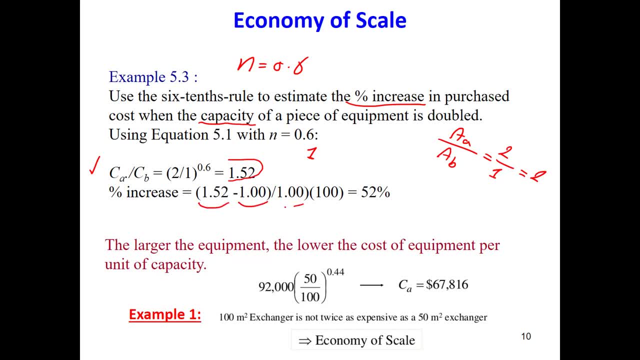 The new value minus the previous value, The previous value divided by previous value times 100, that gives you 52 percent. So when we for that equipment- if I for whatever equipment it is that I don't know that the power is 0.6, if I double the capacity the price will increase 52 percent. 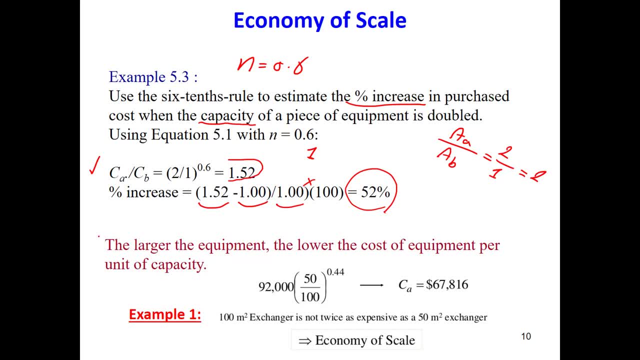 The important, the important message of this example is that if I double my capacity, the price of equipment, it doesn't increase it necessarily two times. okay, It only increase 50 percent. it doesn't increase 100 percent, right? 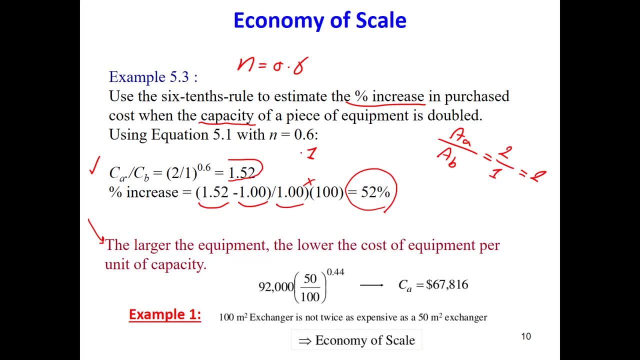 It doesn't get doubled. So that means they have that, that, that the reason is because the cost, the cost and capacity, they had an exponential. exponential relation, okay, not a linear relation. So and we can say in general: 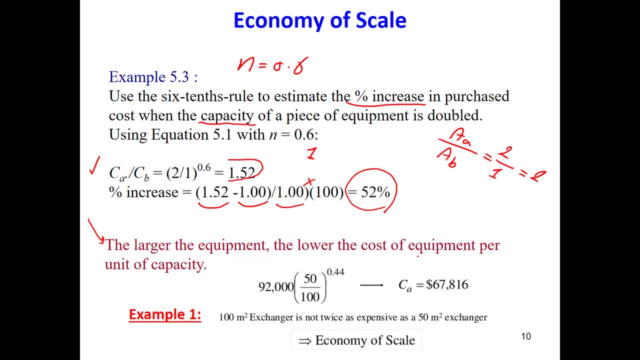 We can say: the larger the equipment, the lower the cost of equipment per unit of capacity. okay, So when we increase the size of the equipment, the capacity of the equipment, the cost increase, but the cost per capacity is less. okay, 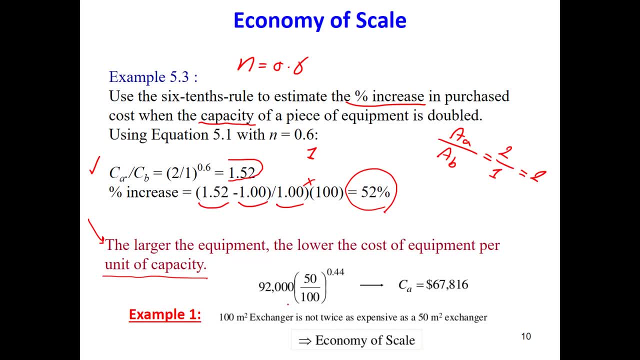 The cost per capacity is less. So here, for example, if I have a equipment, Okay Okay. So if I have a equipment, let's say the exchanger, previously it has it had an area of 100.. 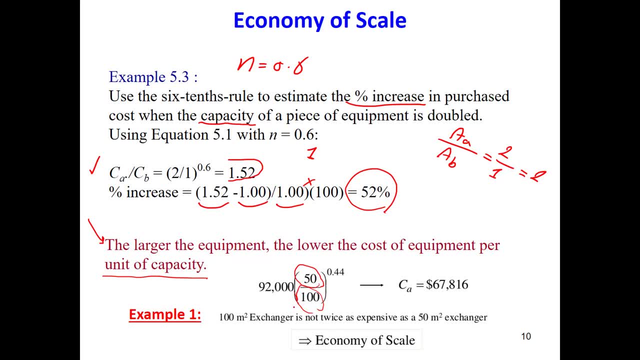 Now I want to build a heat exchanger that has the area of 50. The previous price was 92. If I, if I, if I make the area of the heat exchanger half of the initial area, the price doesn't get necessarily half okay. 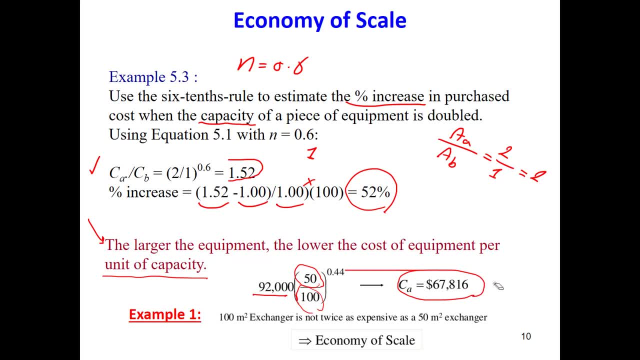 The price decreased, but it doesn't get half. Okay. Or vice versa: If I increase the area, the price doesn't get double. Okay, It increased, but it doesn't get double. So that is called the economy of. we call it the economy of escape. 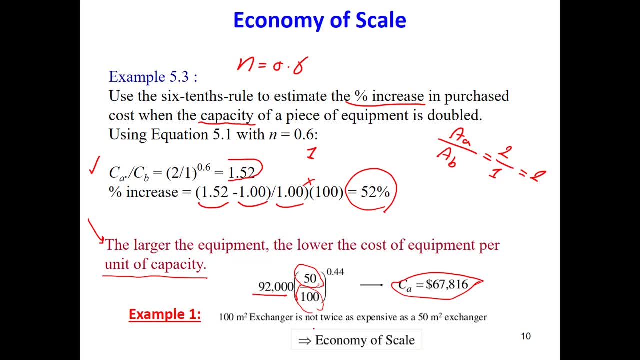 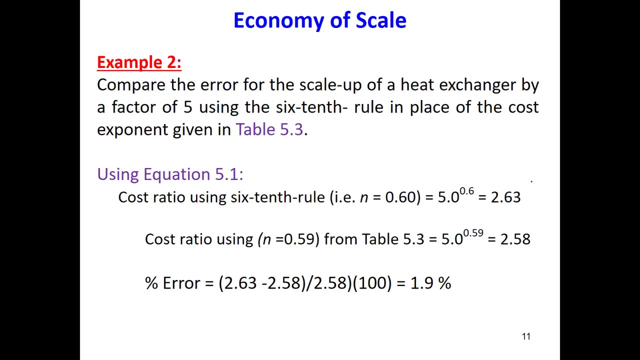 Okay, A 100 square meter heat exchanger is not necessarily twice as expensive as a 50 square meter, based on what you see in this equation, Okay, Okay, Then okay. example two: Compare the error for the scale up of: okay. 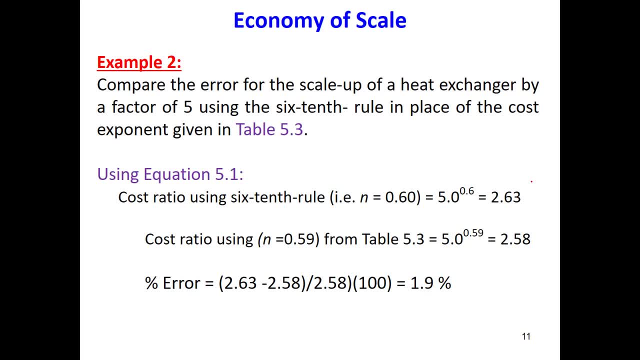 Okay, So compare the error for the scale up of a heat exchanger by a factor of 5, using the SysOCam systems rule in the place of cos exponent given in table this Okay, So compare the error in the scale up of a heat exchanger by a factor of 5.. 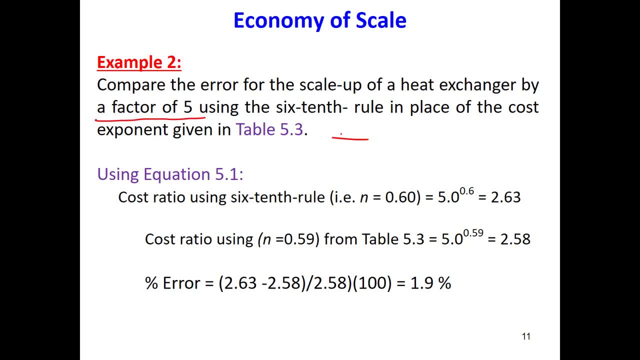 Okay, So you want to scale up a heat exchanger by a factor of 5.. So the new area, the new capacity or the new area? Okay, So the new area, the new capacity or the new area is 5 times bigger than the previous. 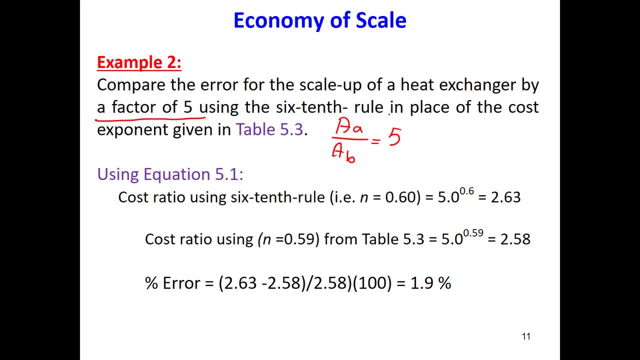 one, Okay. So he is asking you: once use the 6 tenths rule. Okay, It means once use n 0.6 and once go to table 5-3 and find the n from that table. Let's go to that table to see what we have. 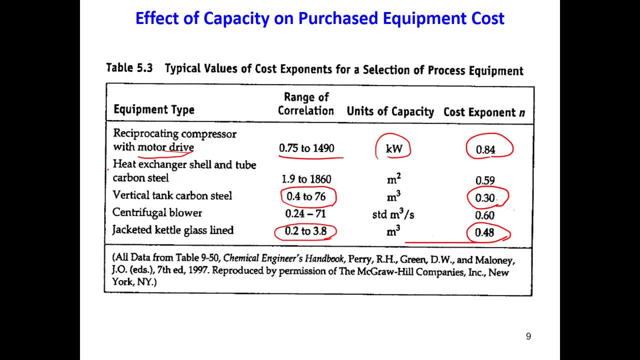 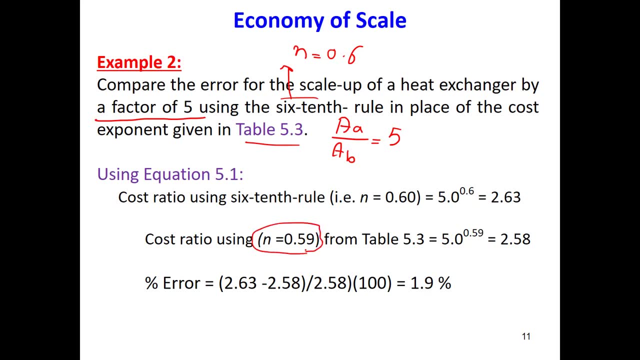 Okay, From that table for the heat exchanger shell and tube carbon steel. for this capacity, n is 0.59, a little bit less than 0.6.. So once we have to use 0.6 and once we have to use the value from the table. 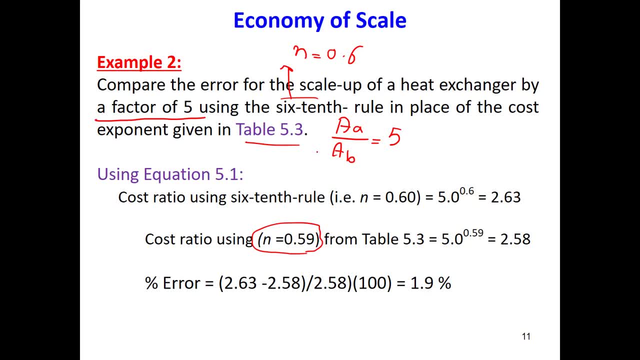 If I use, if I use the one, 0.6,. so, and then I use this equation, the cost ratio, which means CA over 6.. CA over CB, If I use 0.6, I have the area, the ratio of the area power, 0.6, it gives me 2.63.. 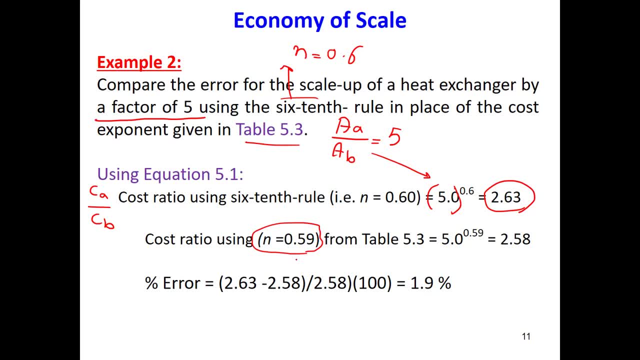 This is the cost ratio. Once if I go use the one which from table, which is a bit more accurate, I will get 2.58,, which is not a big difference. Right, This is 2.58.. It's not much different from this one. 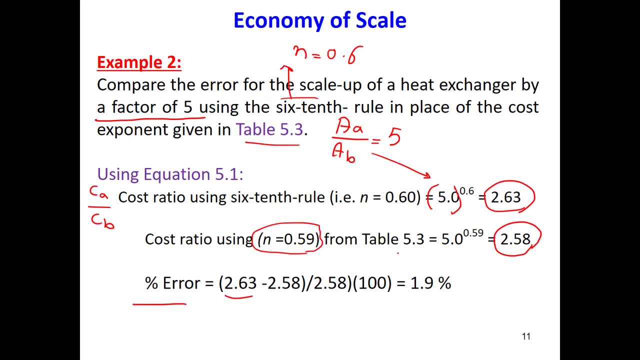 The error between these two calculations. how much the new value, the value from 0.6 minus the value from 0.59, here divided by value from 0.59.. That gives you almost 2% error, which is really acceptable. 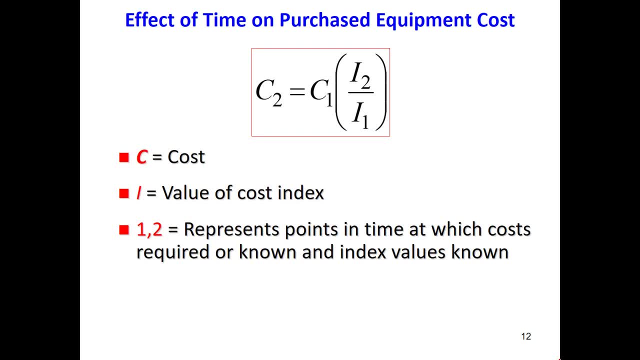 Okay, Another factor that we have is effect of time: Okay, Effect of time on the purchase of equipment. Okay, Effect of time on the purchase of equipment. Let's say, I buy a heat exchanger in 2010,. the price was 1000.. 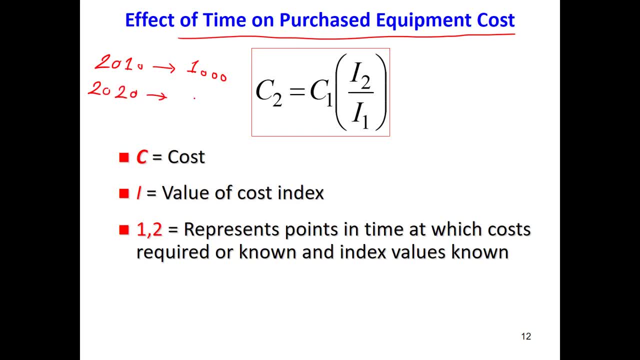 Now in 2020, if I want to buy the same heat exchanger, what is the price For this? we use such an equation, Okay, And we need to use the sum index, Or value of the cost index that we showed with I here. 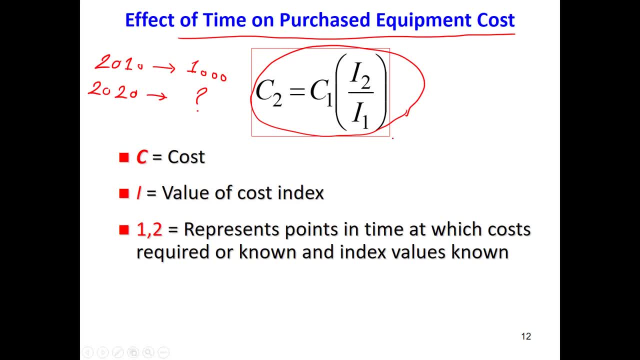 And there are some tables that they give us this kind of index. Okay, There are some companies that give us this kind of index. What is C1 here? C1 is the price of the equipment at 2010.. C2 is the price of equipment at 2020 that we want to find. 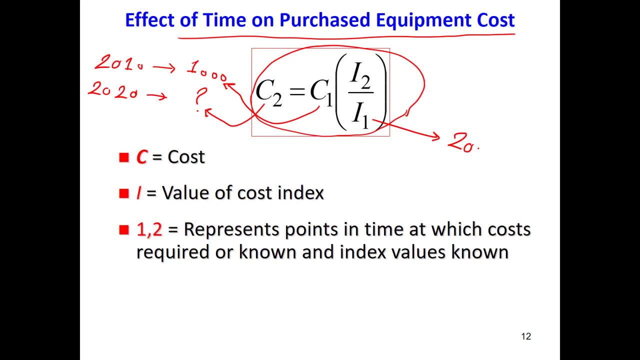 I is the index that in 2010 I won. I2 is the index in 2020, the price index that we will find it from some tables, some resource that they can provide us with this type of indexes. All right, So we have. so we have cost. 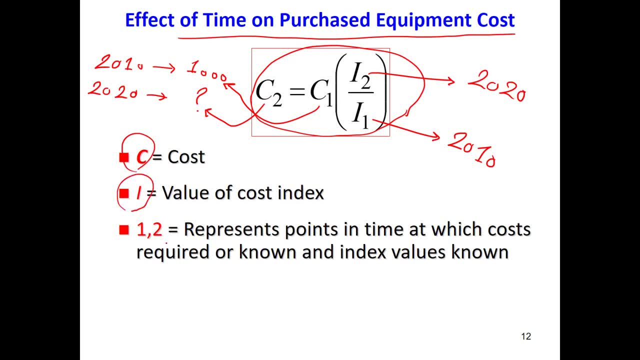 Okay, C is the cost, I is the index, And 1 and 2, they represent the time, the year, that we have to go find the index for that year. So we will see some examples together how to use this index. 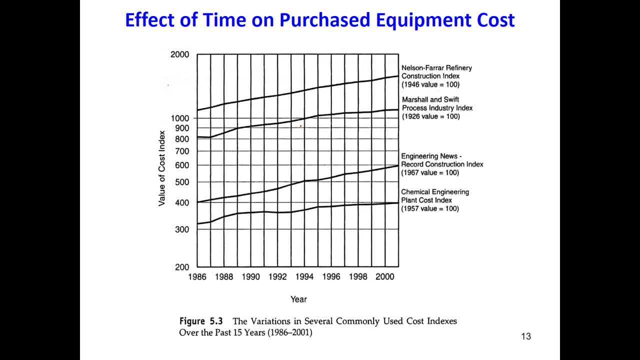 From where we can find this index We have. there are different sorts for the index. There are some companies and some, let's say, engineers that they can provide us this type of index. Some of the famous ones are Nelson-Ferrer Refinery Construction Index. 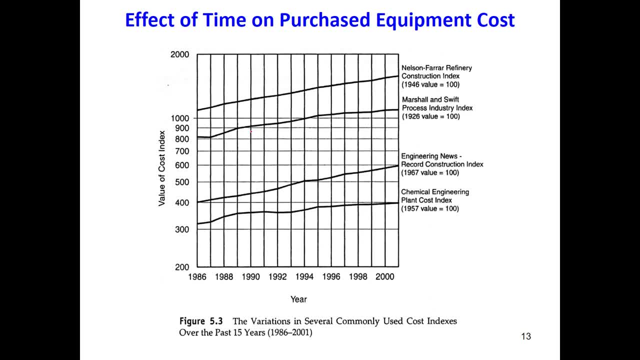 Okay, For refinery we use you know like they, you know they, you know they, you know they listed all those index the I in different years, So you just need to go see in which year you want and then you go find your index. 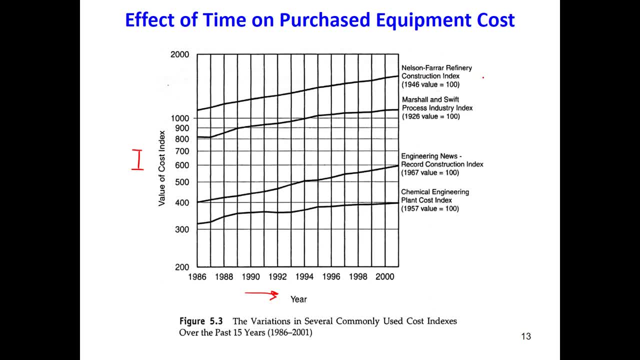 So like we have Nelson-Ferrer Refinery, Ferrer Refinery Construction Index, Okay That the reference value at 1946 was 100.. We have Marshall Swift Process Industry, We have Engineering News Record Construction Index And also we have Chemical Engineering Plant Cost Index. 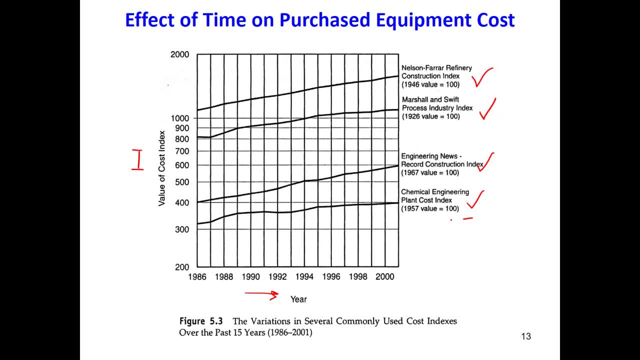 This is the- I mean this- the last one. this is the most useful and reliable index that we need that most of the plant, most of the companies in plant construction, they will use. Okay, Then okay, so you will see some of them here in the next table here. 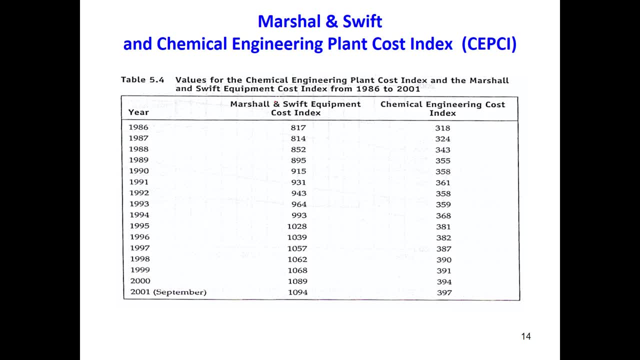 So so Marshall Swift, so the same thing that you saw in the figure, we can have it in tables like that, Let's say from 1986 to 2001.. So, for example, those are the Marshall Swift Equipment Index. Cost I for Marshall. 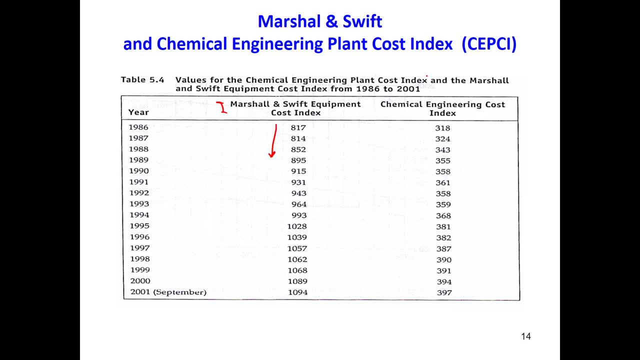 This is for Chemical Engineering Cost Index, Chemical Engineering Plant Cost Index. We just we also show it with CEPCI. You will see a lot of abbreviations like this. but, as I said, don't worry, don't panic, There are just different, different abbreviations that you need to kind of know and use this. 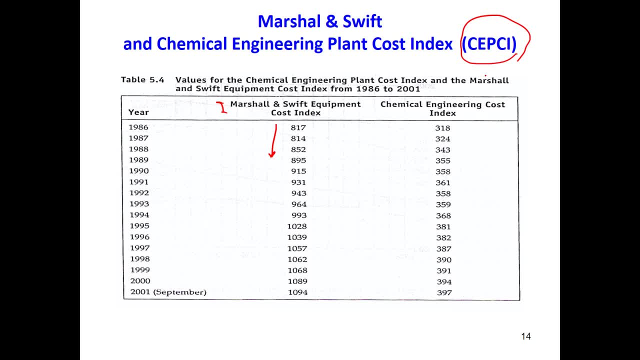 in this course. Then we have: okay, we have Marshall Swift Chemical Engineering Cost Index. Marshall Swift Chemical Engineering Plant Cost Index, CEPCI Then okay, so this is for CEPCI Index, This is Marshall Swift. Those are- both of them are kind of used, but the Chemical Engineering Plant Cost Index. 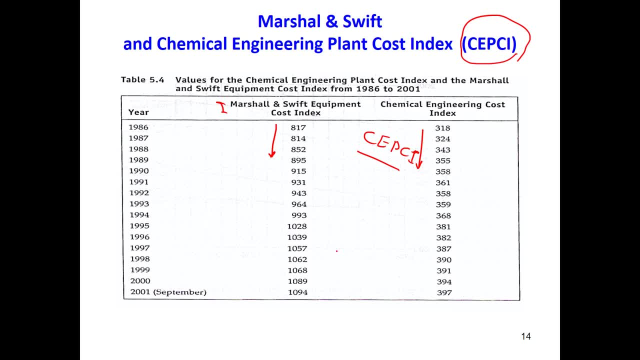 is more useful. So this is generally for a plant okay, for a major equipment of a plant Okay, But there are some tables that gives us such an index okay. If I mean there are some tables that is also published, I mean that is also related. 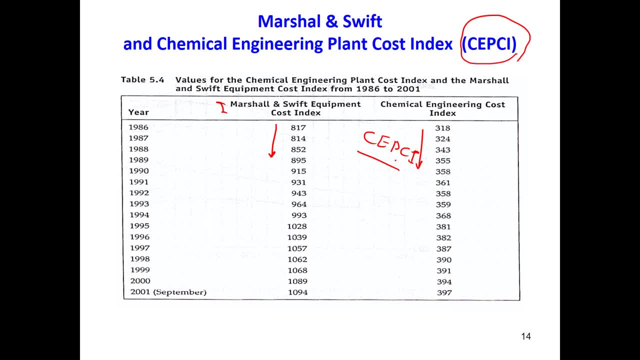 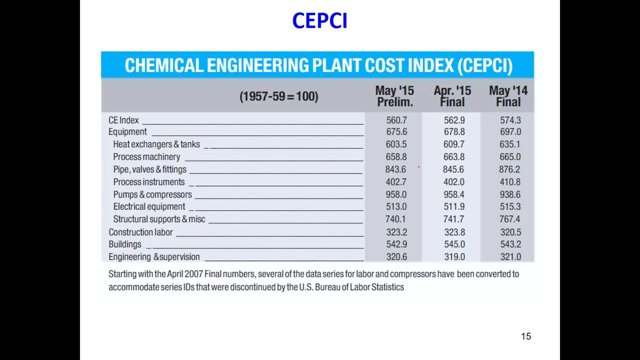 for Chemical Engineering Plant Cost Index, CEPCI, that give us the value, the index for a specific equipment. okay, for a specific equipment, Let's say for heat exchangers, For machinery, for pipes, valves, fittings for pumps, compressors, okay. 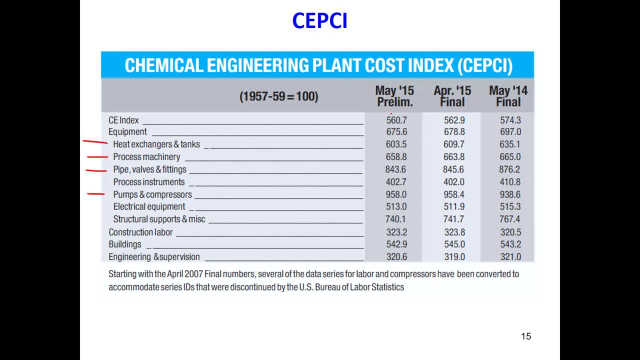 So they give us a specific for that equipment, that they even list them, sometimes month by month, you know like, sometimes by. you know like every month those index, those index are reported okay by some companies. Okay, So let's say, in May 2015,, in April 2015,, May 2020, we have all of them, especially 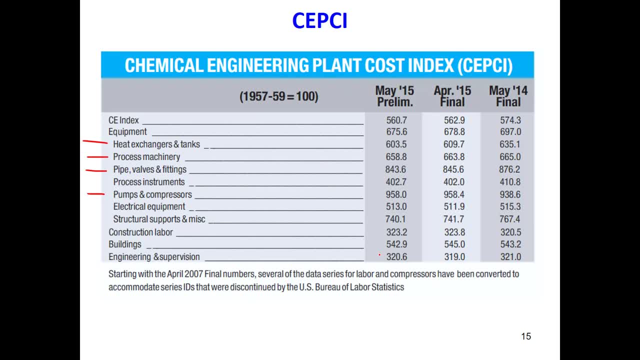 now, you know, like that we have this crisis because of the virus, that many economies are down. you know, like we had a big drop in the stocks, So there are a lot of economical issues these days because of this issue that is created. 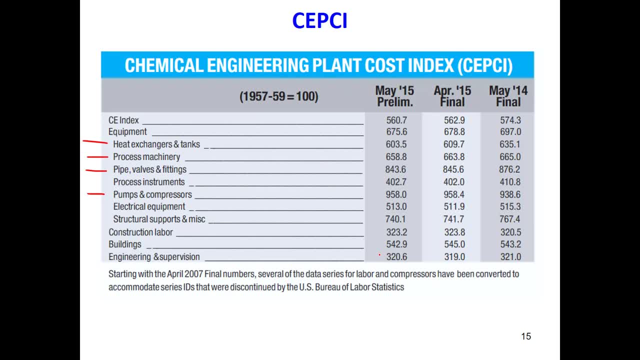 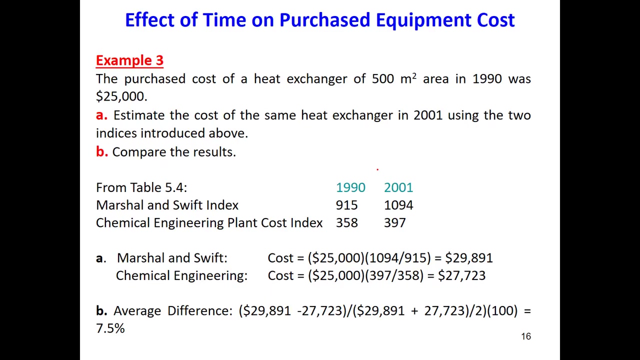 by the virus. But that you know, like the like, for sure, like the companies who are producing this index, they will, they will report soon. you know how this index they have changed. okay, because of the change in the stock market and, in general, the economy, the global economy. 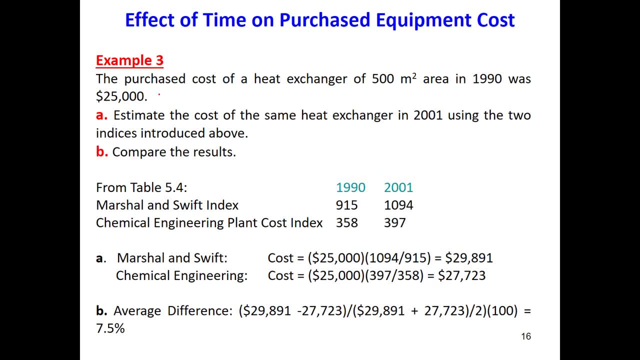 Okay, Let's see how we use this type of index: The purchase cost. one example: the purchase cost of the heat exchanger of this area In 2000,. in 1990 was 25,000.. So we have the area of the heat exchanger, the year, the year. this is my first index. 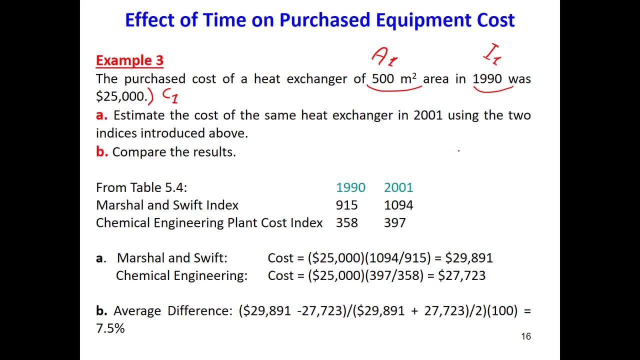 and the cost: C1.. All right, So estimate the cost of the same heat exchanger in 2019.. Okay, In 2000,. 1. We want C2 in 2001.. Okay, And compare the results. 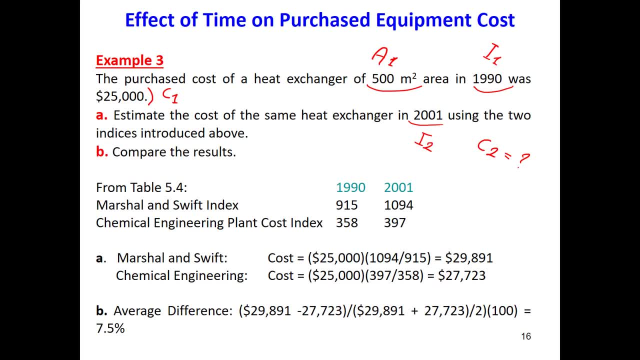 How we will do it. So let's do it. Let's use both Marshall and Swift and CPI, the chemical engineering plant cost index. Okay, CPCR. So let's go to table 1990 and 2001,. right, 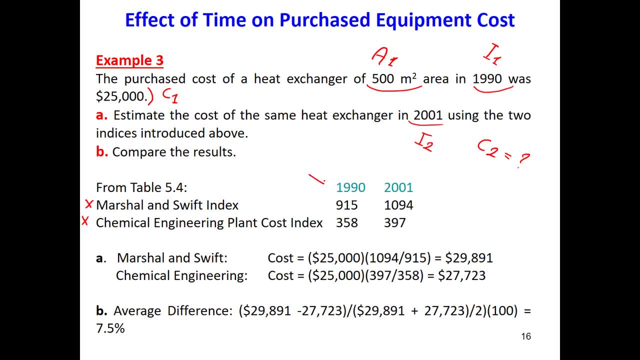 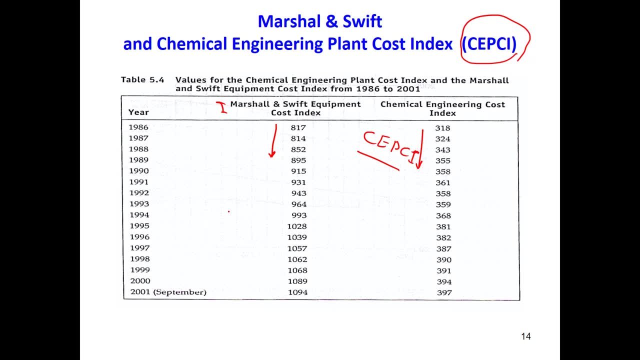 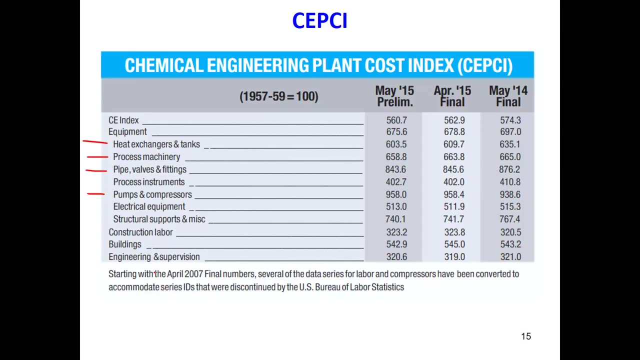 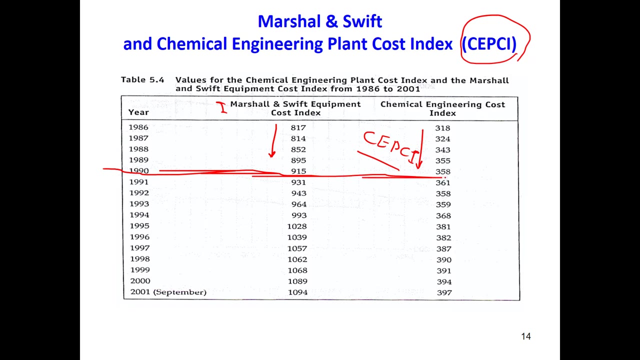 1990 and 2001,. here Let's go to table 5. In slide 14. 19, let me see: Okay, 1990 and 2001.. 1990 is here. Okay, 1990 and 2001,. here 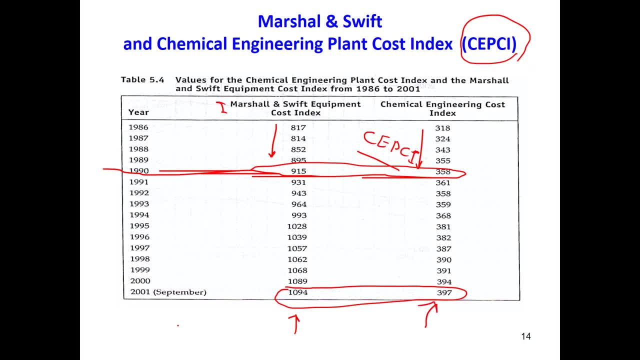 We will use both Taylor Swift and chemical engineering index. Okay, So in 1990, for this one is for Taylor Swift- is 915 and 2001 is 1094.. For chemical engineering index is 1990, 358 and 2001, 397.. 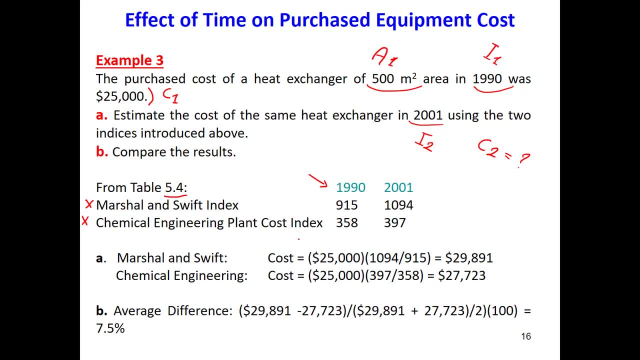 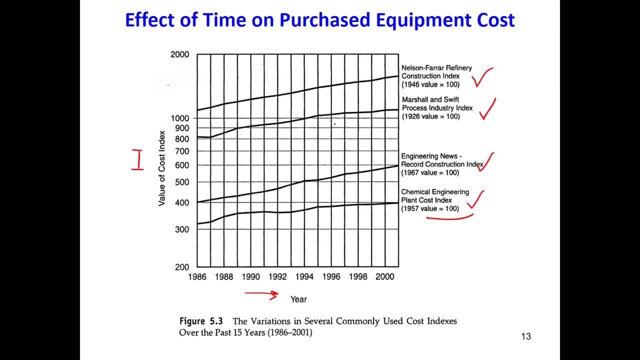 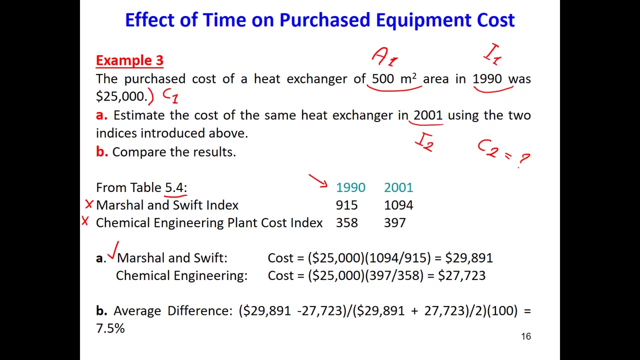 Okay, So this is how I listed my index for Marshall Swift and chemical engineering, So let's do it for Marshall Swift. We will use this equation right. This equation: C2 is equal to C1, I2 over I1. 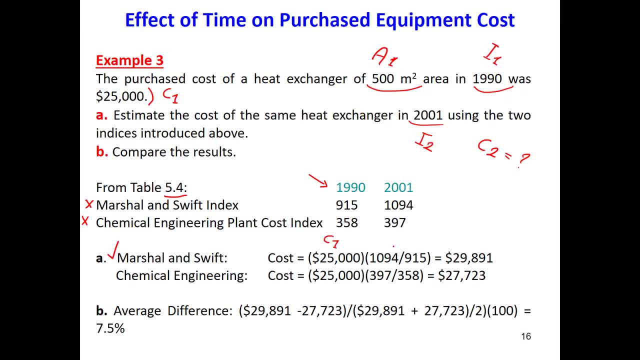 So initial cost: C1.. I2 in 2001 for Marshall Swift and for chemical engineering. The same thing for in 2001 and 1990.. The same thing for chemical engineering. You will get these two values for your cost. 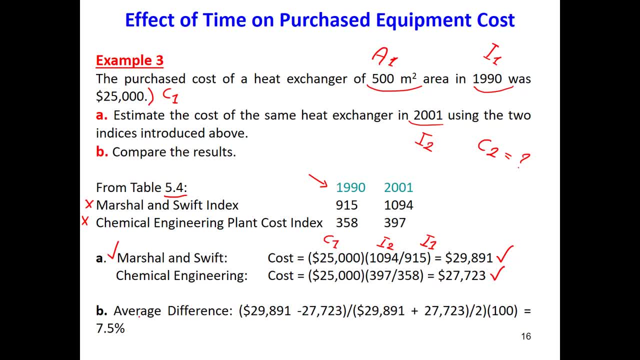 So how much is the error between them? I mean, we will use the average difference. How we do it? We take the average of these two values here, These two values divided by 2.. Some of these two values divided by 2.. 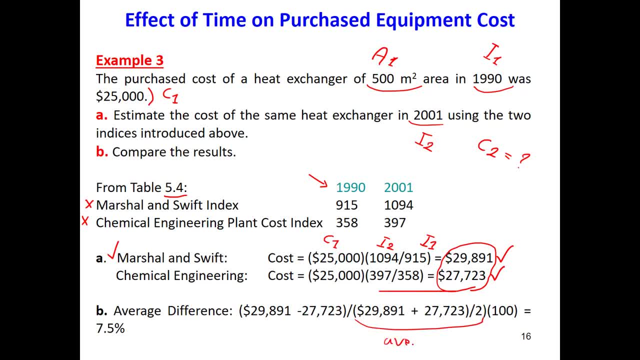 This is how we find the difference. So we take the average of the two values from the two metals. Then what we do? We reduce the Marshall Swift from the chemical engineering divided by the average times 100.. The error is about 7.5.. 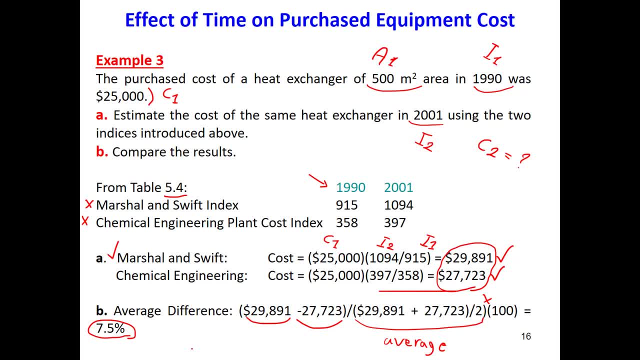 7.5%, Which is not a bad error. Below 10% is always a good, acceptable error. So this is how we use this equation. Now we will have also one example that we will consider both the effect of capacity and the yield. 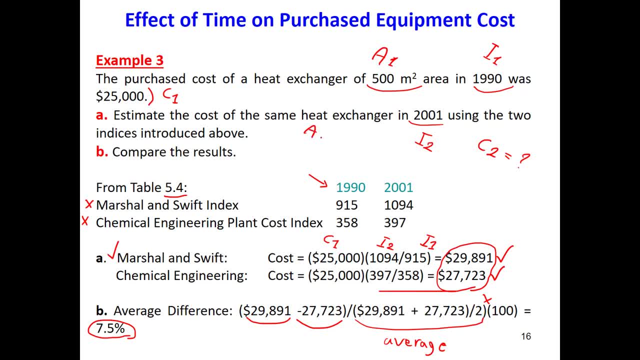 Let's say now, if I ask you what's the price of a heat exchanger that has an area of 1000. Let's say 1000 cubic meters in 2001.. So how you will calculate it, You have the cost for this heat exchanger in 2001.. 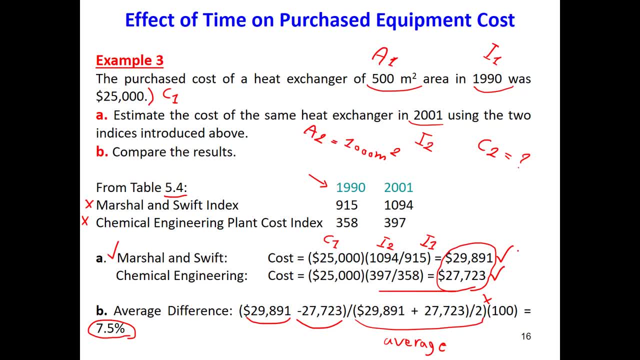 You have the cost already calculated, Then you have to go one additional step and consider the effect of capacity A2 over A1. Then we will use the equation that we have, The cost index, The, The, The Exponent 0.6 that we use. 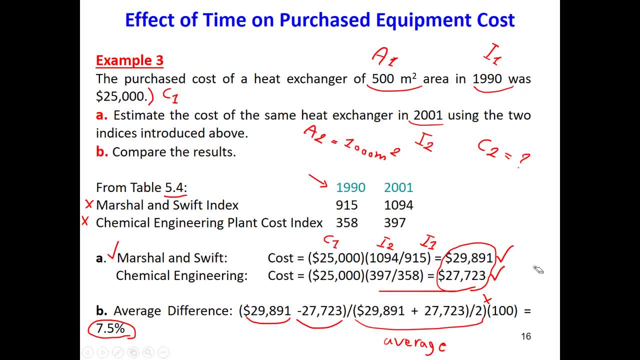 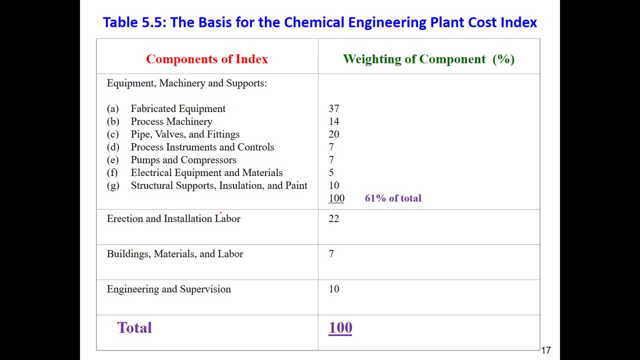 Okay, So you will see that in the next few slides- I think the next few slides Okay. Like this table, it shows some kind, Some ideas about the cost of the chemical plant. Okay, I mean, like how this plant index they are calculated. 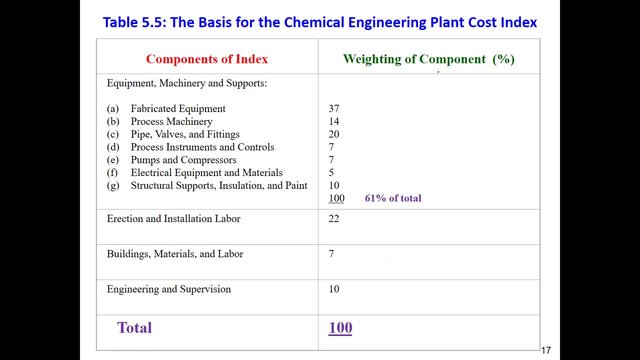 Let's say, for the heat exchanger that we have, Let's say in For any equipment, that Let's say in 2001, I have the index 105 and in 2020, I have 215.. How these values are calculated. 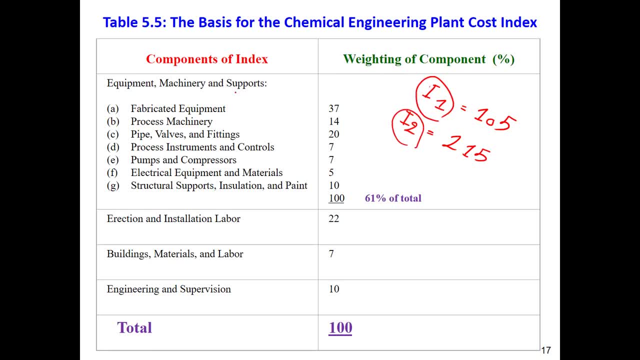 When they are How these index are calculated. When they are calculating the index, they consider the contribution of each work that has to be done on the equipment. Okay, Each work, The Each of the work that we will put to build that equipment, that have several works to 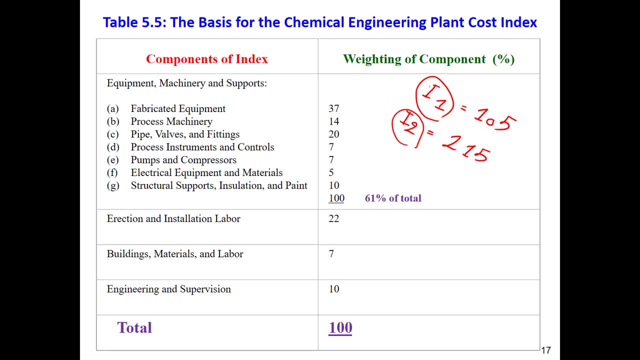 be done is Has some contribution in the total price That usually they categorize it in this way. This is one sample. Let's say the fabrication of equipment. it cost 37% of the total cost of equipment. Machinery is 14%. 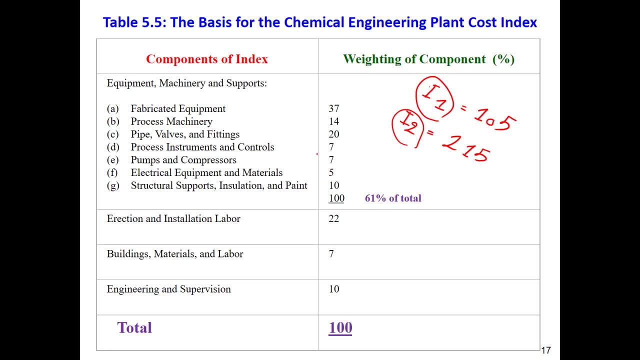 Piping: 20%. The instrumentation: control: whatever we need to put, 7%. Okay, If we need to put some compressor pumps, whatever it is 7%. The electrical works need to be done. materials: 5%. 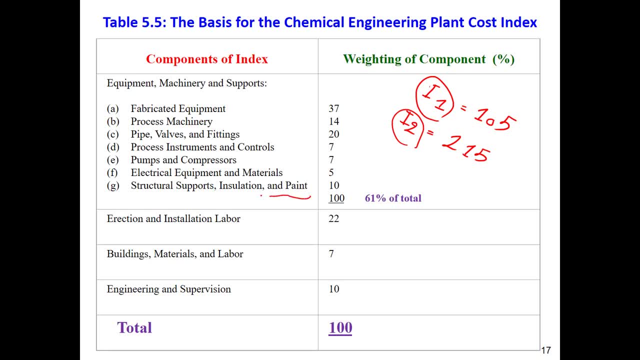 The isolation painting. that is something very important. This job is 10%. Then labor installation labor: 22%. Labor building materials- you know some other stuff that you need to spend- 7%. Supervision engineering work: 10%. 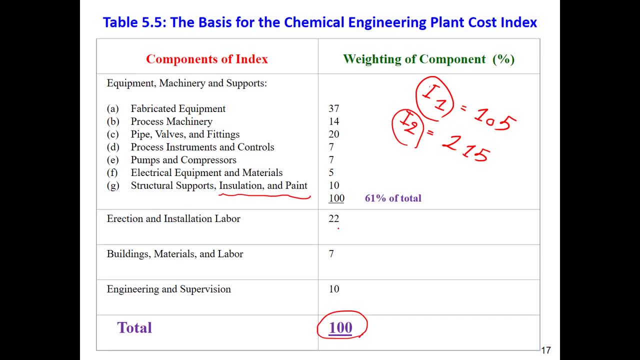 Totally. this will be the totally 100% of the price of that equipment. When they are calculating such index, they will do it usually in this way That they will find the contribution on which of the price, and then they will do some additional. 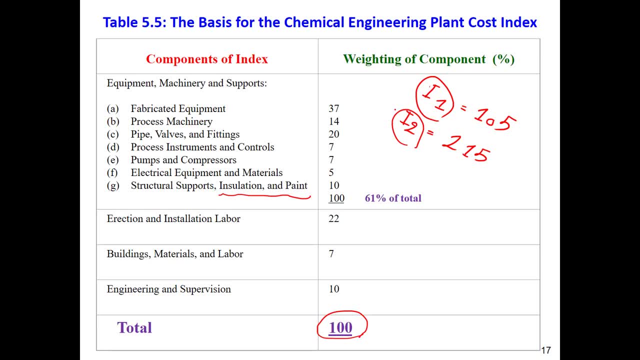 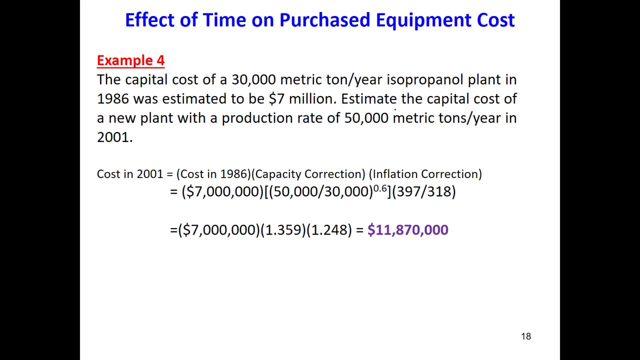 calculation to find these indexes. Okay, so now we are going to talk about this example. as I said, how to consider the effect of the capacity and time together. The capital cost of 3,000 metric tons per year isopropanol plant in 1986 was estimated. 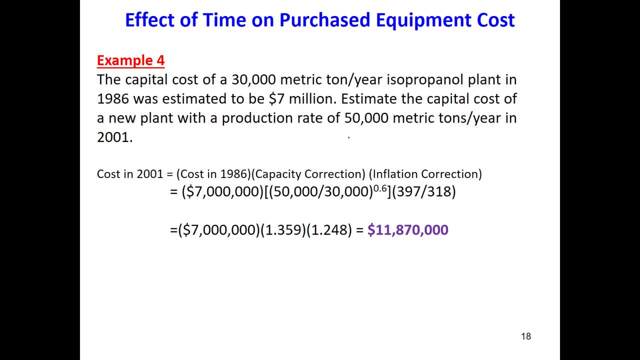 this much Estimate the capital cost of the plant that has the production rate. this in this year. So what we have in 2000,. in 1986, we had a plant with this capacity. The price was $7 billion. So this is my year, my capacity and my price. 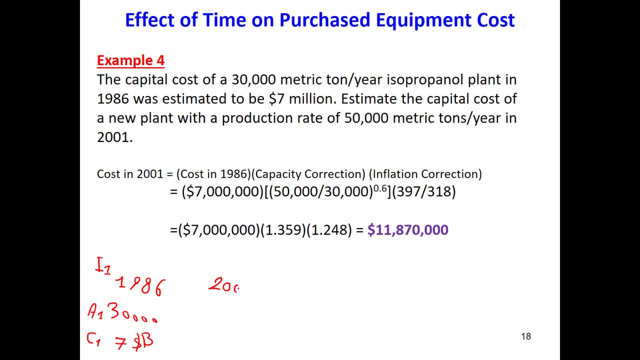 Now you are asked: in 2001,. in 2001,, which is the new year, I mean the year that you want to calculate the price. I don't know what's wrong with this. Okay, in 2001,. this is my index 2, for the new capacity is 50,000, A2, I want to find. 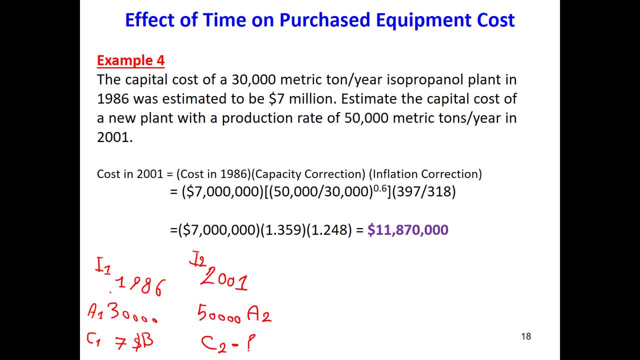 the price. All right, so I will use for the price I have to find the index. Okay, So let's use the engineering chemical engineering index. Let's see in 1986 and 2001,. what are the engineering index? 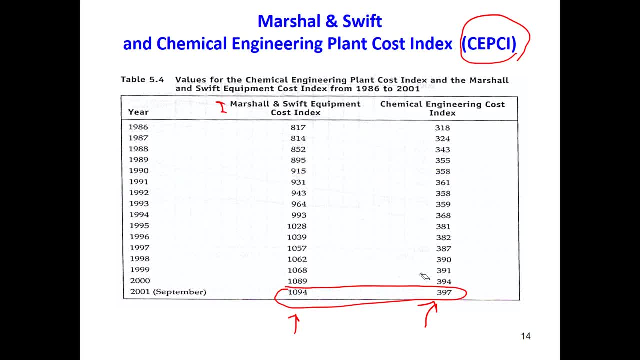 Okay, let me clean up this a bit. So in 1986 is here, the index is 318.. In 2001 is 397, 318. And 318.. Okay, 397. 318. 397.. 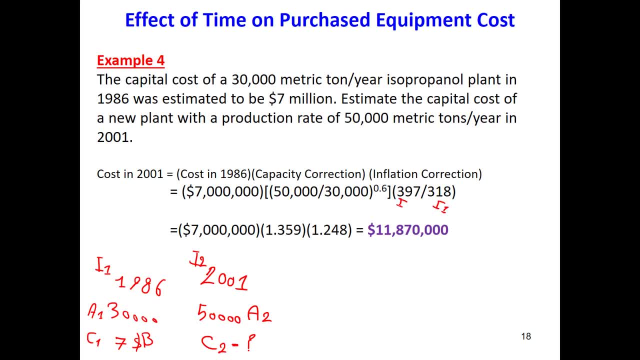 This is my index. So what I have to do here, I want C2, which will be C1,, I2 over I1, this is the effect of the year, And I have to also consider the effect of capacity. So C2 over A1, divided by use the six-tenths rule. 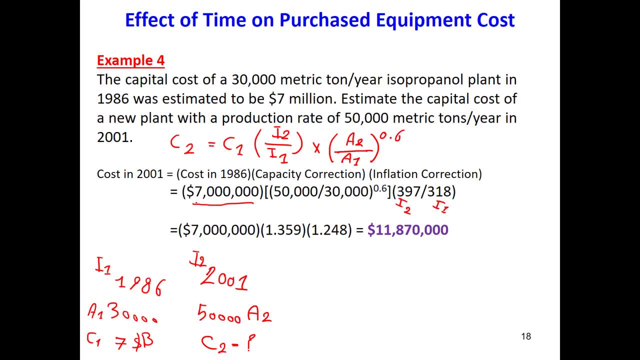 Okay And fine. So we have the first price, which is 7 billion dollar, The new capacity, okay, which is 50,000 divided by previous capacity power, 0.7.. The index in this year, in 2001,, is 397.. 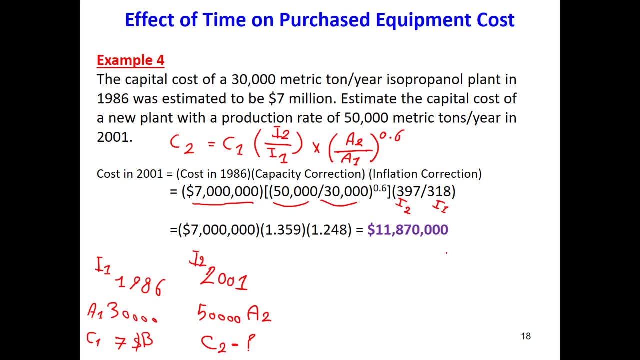 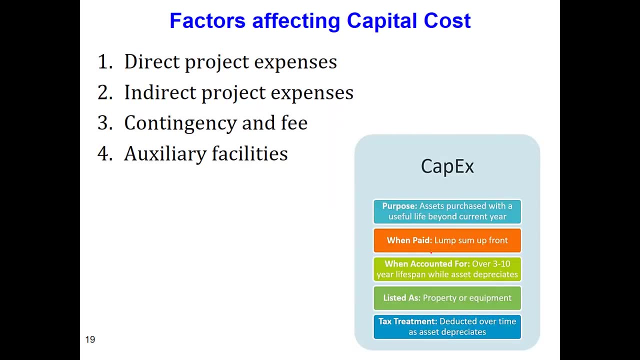 And the previous index is 318.. So if you do the calculation, you will find 11, almost 12 billion dollars. So this is how we solve this equation. Let's say this example: Okay, Factors that are affecting the capital cost. 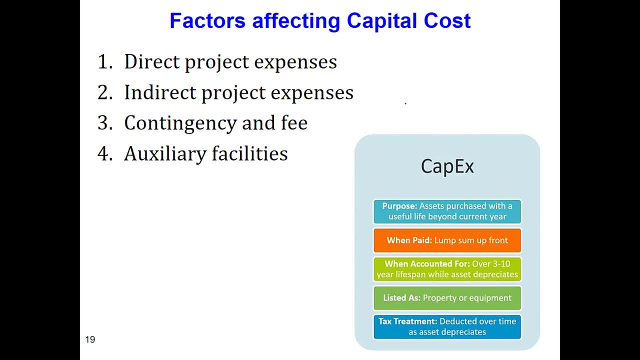 Capital cost and interest. Capital cost it means the total cost of construction of the plant or equipment. So we consider we have different type of, we have different type of different type of expenses, that we categorize them usually to this list that you can see here. 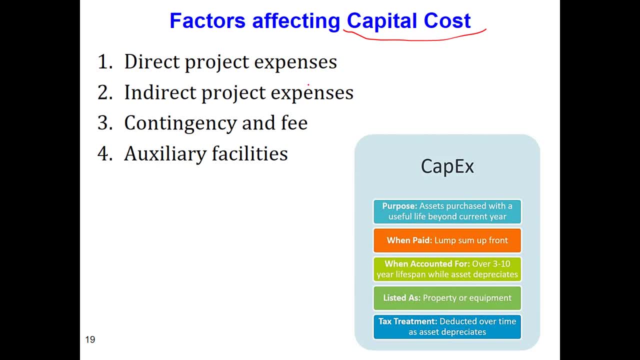 We have direct project expense. Okay, We have direct project expense, indirect project expense, contingency and fees. Like contingencies are like those expenses that we might have in future. You know, it can be any, like some I don't know, some disaster, some accident, some. 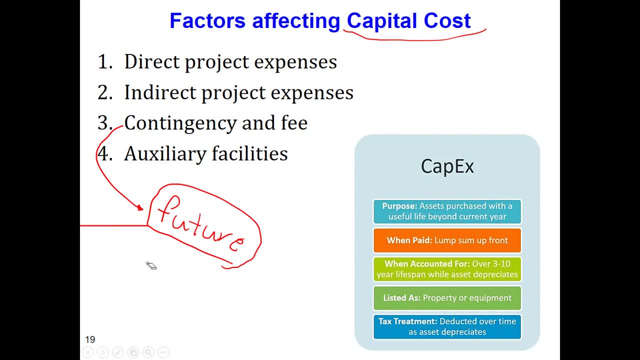 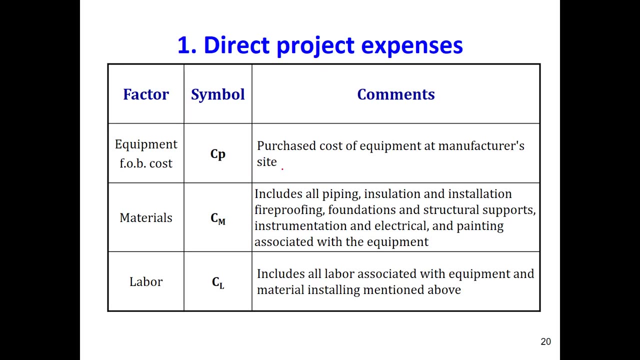 some expenses that we cannot really predict, Some, some other fees And auxiliary facilities, Let's say utilities that we need to build to, to operate the plant. So let's say let's start with each of them and then we will see what are them. 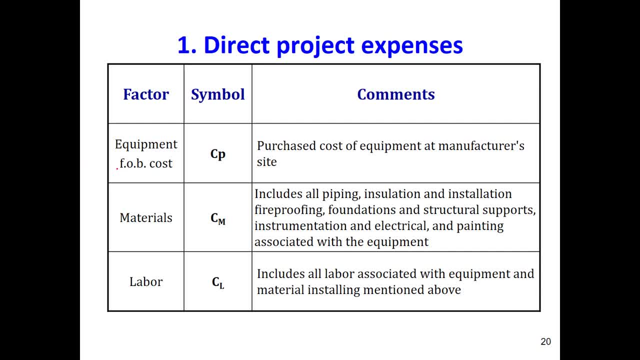 So direct expense are those expenses that you can see: Equipment fabrication cost, Okay. Cost of equipment: Okay. So it's a purchase cost of equipment at the manufacturer's site. Like, let's say, you buy a heat exchanger from a company, then you have to bring that heat. 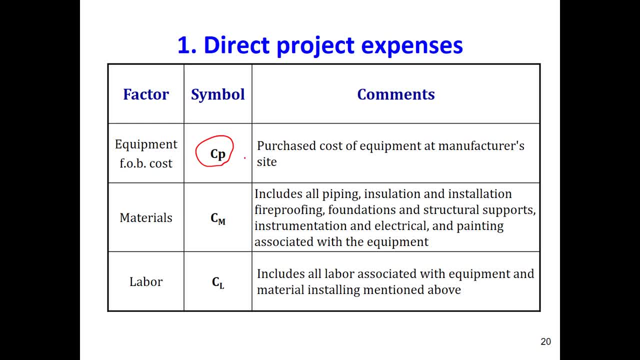 exchanger to your plant. Okay, So this is the price of equipment. CP is the price of equipment in the manufacturer's site, in the company's site. We don't consider in this factor, we don't consider the transportation. I don't know if you, if you have to import it from other country, the taxes that you 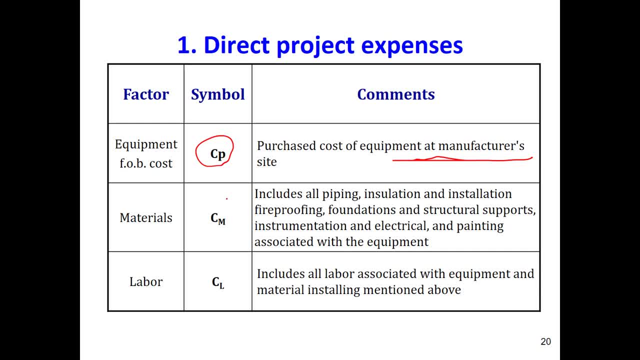 have to pay and some other expenses: Material expenses related to material. we show it with CM. That includes all the piping, isolation installation, fire proofing foundations, structural supports, instrumentation, electrical painting and whatever material that you will consume it. 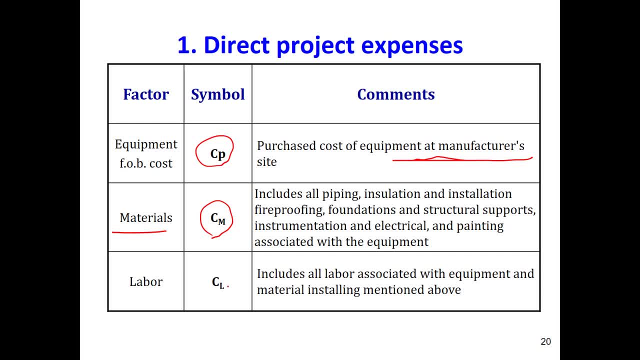 will be considered as direct expense And material expenses. Labor expense: You have to get some labor to do the job for you. Okay, All the labor associated with equipment, material, installing the material you know, like installation, painting, construction, whatever labor you need to do to use this, will be shown in this. 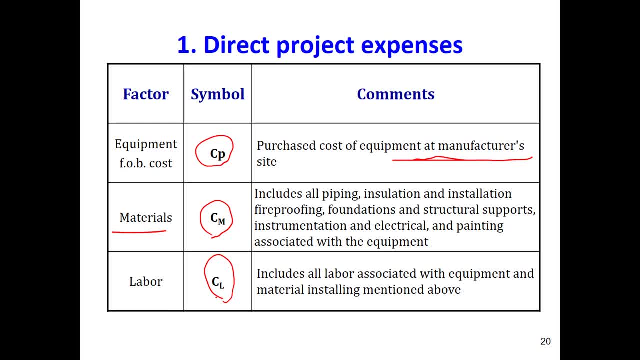 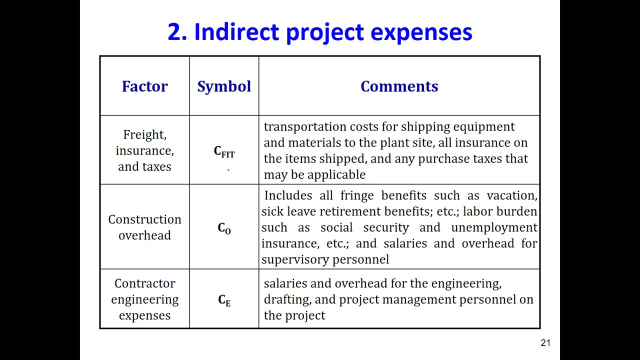 index or indicator that we call it labor cost. we show it with CM, Equipment or process cost, CP. Okay, Those are the direct costs that you have. You have indirect costs. Okay, What are indirect costs? Insurance, tax, transportation, freight. 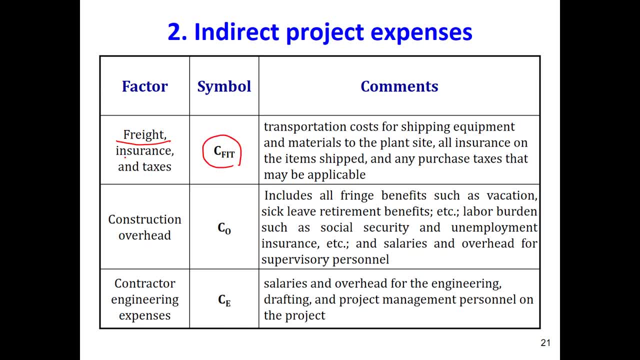 So that we show it with this Freight insurance tax CFIT. those are the. this is considered as indirect cost, which is the cost related to transportation. Okay, Shipping of the material from the manufacturer to the plant. size, Insurance that you need to pay for the equipment to ship it. 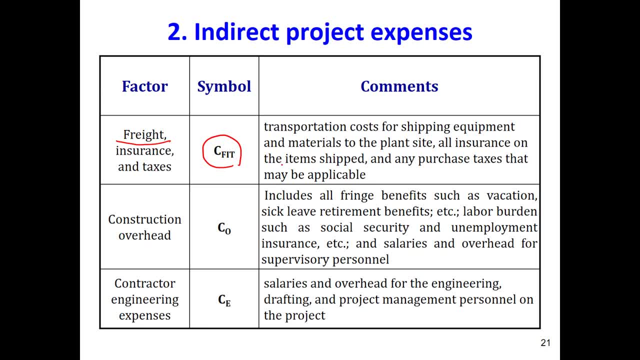 Okay, Because even the shipping- when you are shipping something, there are expenses with it And any purchase tax that may be applicable- Okay, Any purchase tax That will be that might be applied. Okay, There are always taxes from when you buy something from other countries. 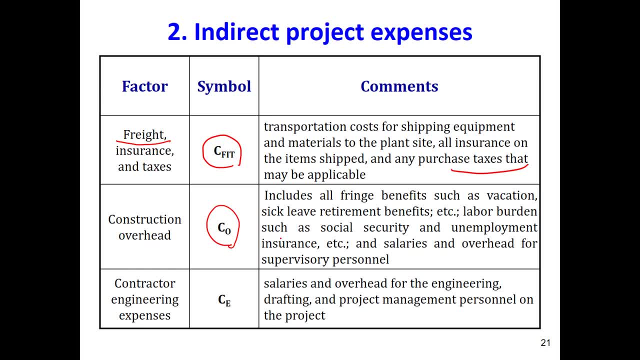 Construction overhead. Okay, So then you know, like always, some overhead or some extra, additional, additional expenses, especially in construction, that you need to also consider. Then we show it with this: CO overhead. This is. it includes all the extra benefits that you need to provide. 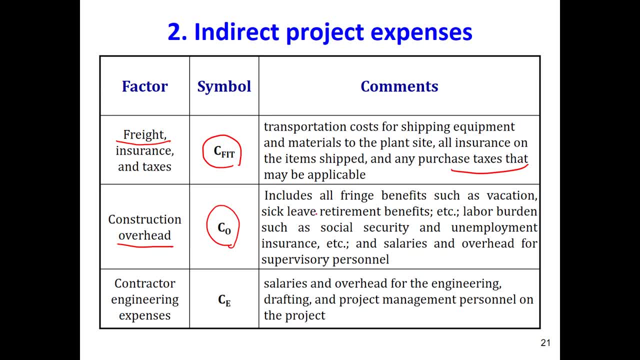 Let's say vacation- There might be some sick leave- retirement benefits- Those are the things that you have to provide for your labor. Okay, Labor burdens such as social security, unemployment insurance. Okay, Salaries and overhead for the, for the supervisor. 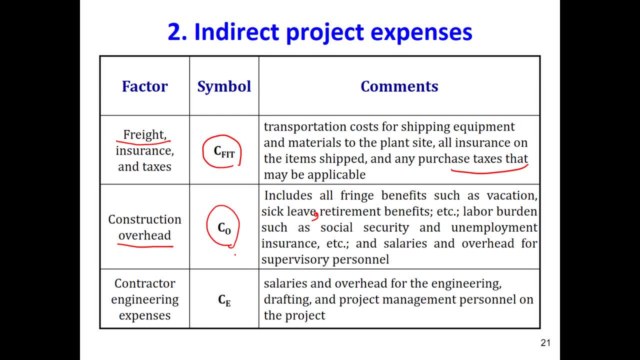 Okay, So there are some overhead expenses, which is mainly related to the labels that you have to also consider Contractor engineering expenses. So, like for each of the job that you will do, you need to have the contractor, let's say, for construction, for installation, for a startup. 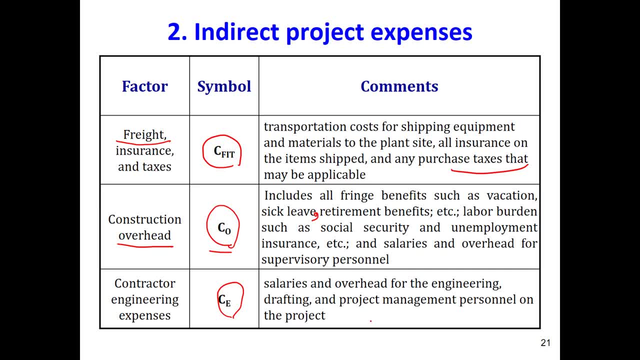 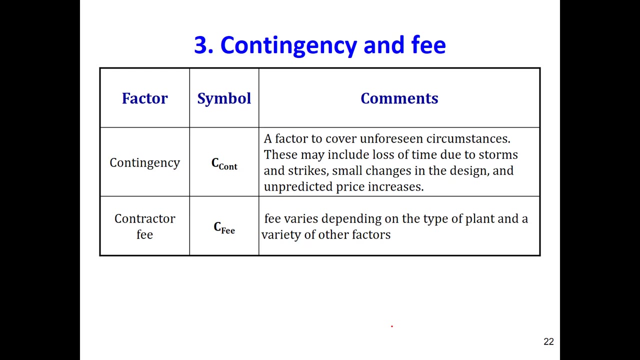 So, like you have to also consider for project management, you have to also consider those, those costs that we call it in general engineering expenses or engineering costs. That is, that includes all this item here. Those are your indirect expenses. We have also contingencies, contingency and other fees. 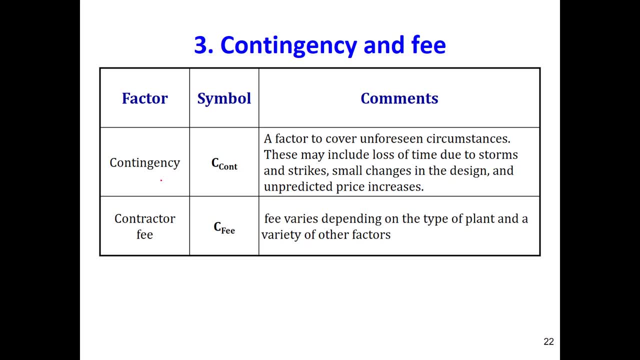 Let's say the fee, that the thing that might happens in future, that we call it contingencies. We show it with this C contingencies. It's a factor that we call it covered any unforeseen, unpredictable circumstances in future. Okay, So it might be, you know, waste of time or lose of time because of a stormy weather or 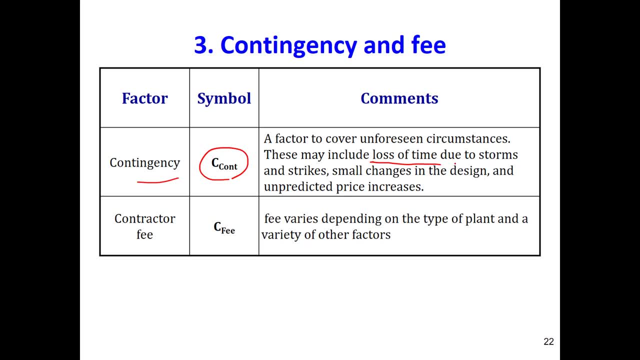 some strikes or labor day strikes all the time in different countries, Or if there is a small change in the design, okay that you do the design, you start the project, you go ahead, but you see that there are some things that need to be improved. 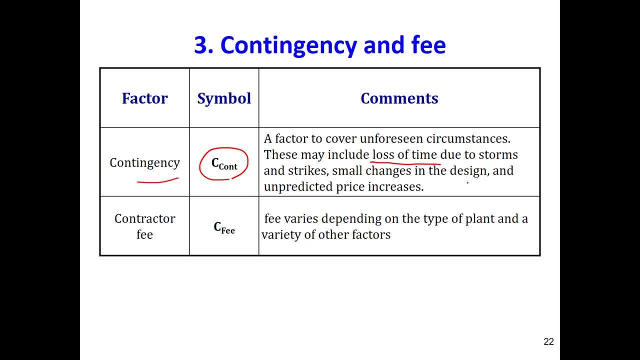 You start the project, you design, you redesign the things and you continue. Okay, So those are unpredictable prices, unpredictable things that you need to consider, or unpredicted price increase. Okay, Like what we see in these days, in this condition that we are the prices, they might increase. 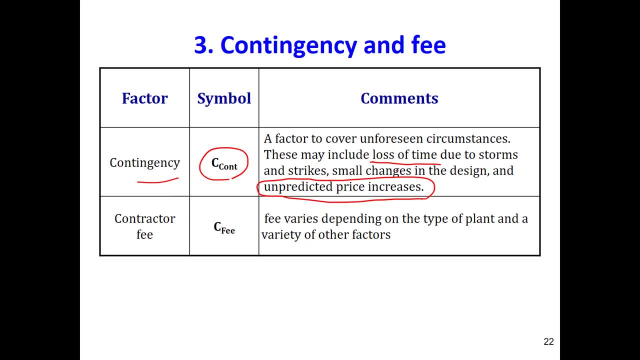 because of We have many issues, economical issues. So those are the things that we all consider in this factor. Contractor fees that we showed with the fee is, you know it's like, depending to the type of the plan and some other factors, you know, there might be some contractor fee that we 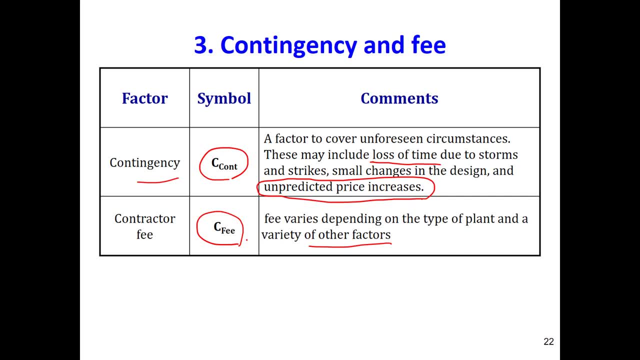 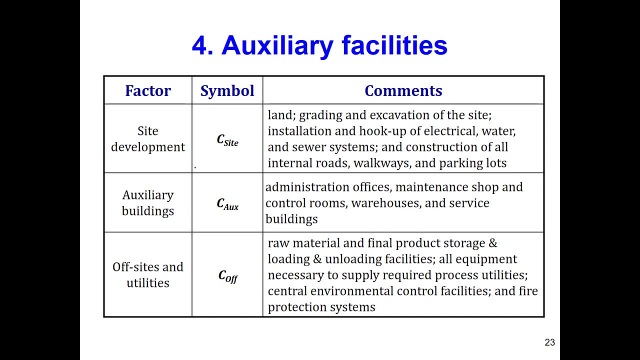 also need to consider. So this is the third part, And last part is auxiliary facilities that we have. Okay, Let's say site development. we showed with C site we have auxiliary buildings, the cost of those auxiliary buildings. we showed with C auxiliary or AOX, and we have off sites and 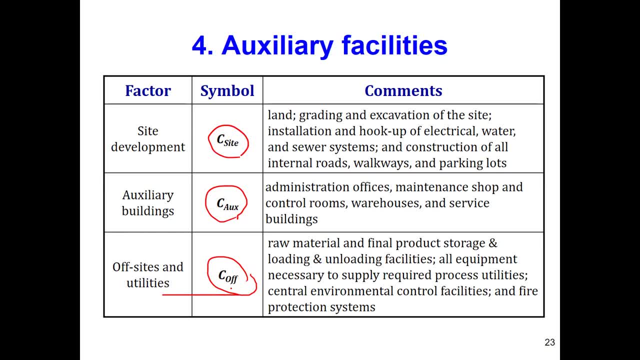 utilities, that we show the cost of those facilities with CO up. Okay, So what is site development cost? is the cost related to the land? Okay, Then grading, grading of the site, grading, excavations of the site, Then installation of some electrical, light water, sewer systems, construction of all. 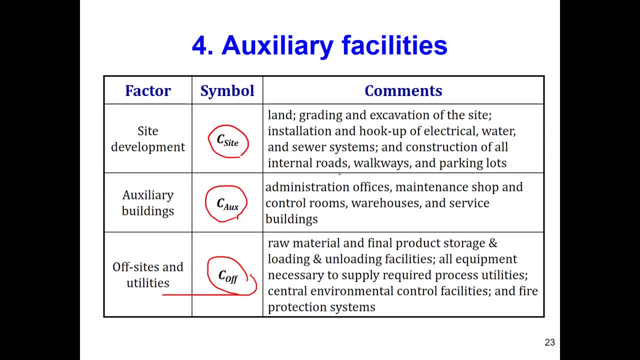 the internal roads that we need to do, walkways, parking lots, so anything, any cost that you need to pay to develop the site. Okay, Then offices, Okay, Okay, So we have auxiliary buildings, So we need to build a building for administrative staff or administration offices and maintenance. 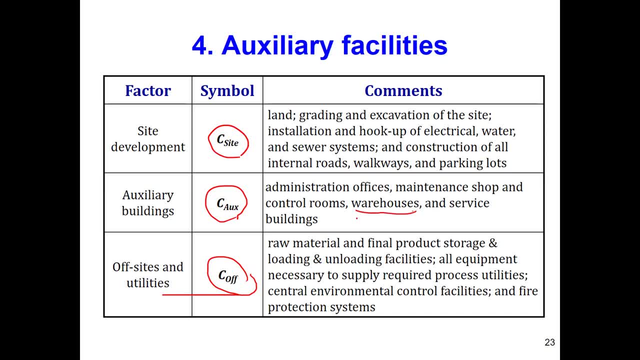 shop storage, control room storage or warehouses and service buildings. So this is some cost that we need to pay. We do this usually in the initial stage of the project. We build the kind of Building We construct a building that is mainly for managing administration, offices, services.